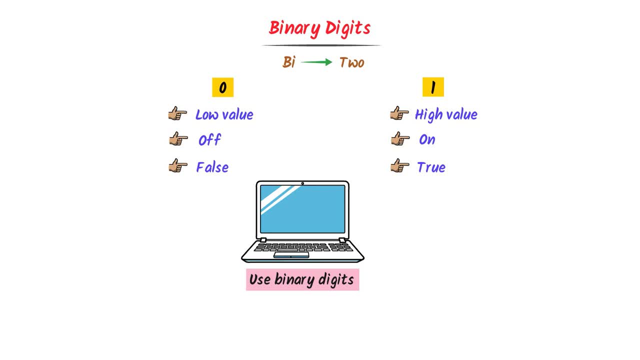 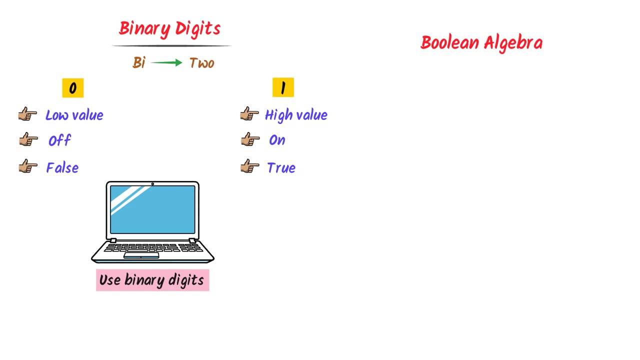 know that every computer use the binary digits zero and one. Now I will teach you the basic concept of boolean algebra. only in one statement, I mean in boolean algebra, we use binary digits and one plus one is equal to one, because there is no other digit. Let me 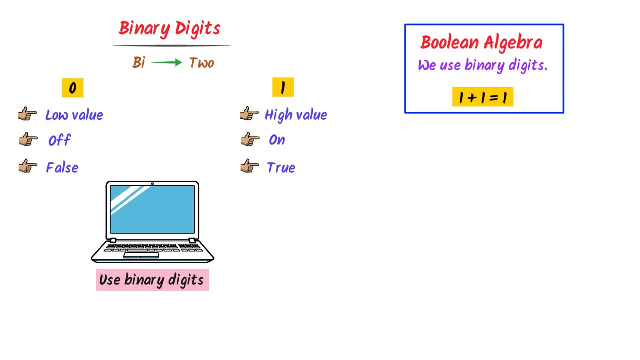 repeat it: In boolean algebra we use binary digits, and one plus one is equal to one, because there is no other digit. Hence, if you learn this basic concept, you can easily learn boolean algebra. For example, consider addition of binary digits in boolean algebra. 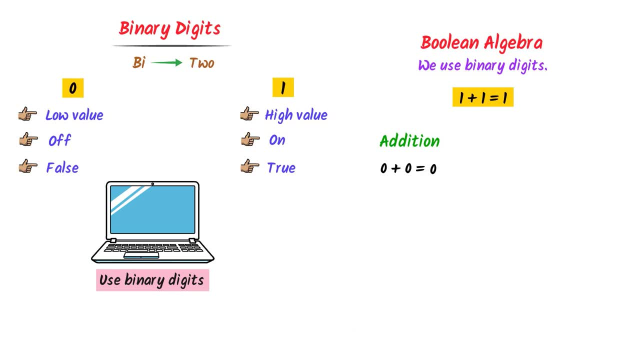 We know that zero plus zero is equal to zero. Zero plus one is equal to one. One plus zero is equal to one. One plus one is equal to two, But in boolean algebra there is no such digit like two, So one plus one is equal to one. Secondly, consider multiplication. 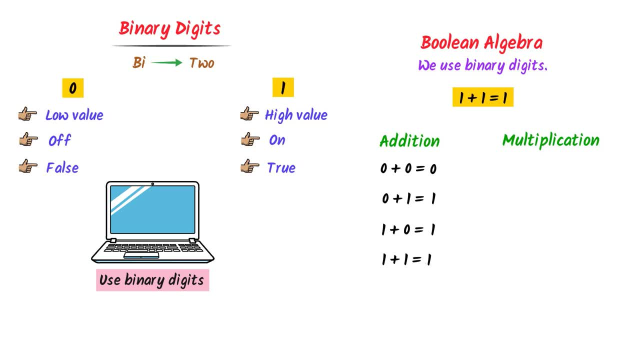 of binary digits in boolean algebra. Remember that zero and multiplication is a hydrogen bomb. It finishes everything. Let me repeat it: Zero and multiplication is a hydrogen bomb and it finishes everything. Like zero and two, zero is equal to zero. Zero and two: one. 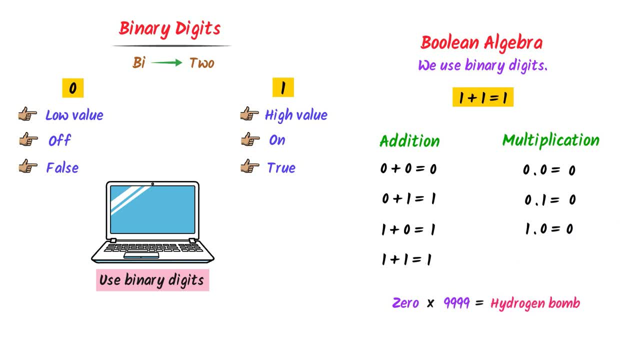 is equal to zero. One and two: zero is equal to zero. And one and two, one is equal to one. Thus, remember that in boolean algebra, all the mathematical operations are the same, except one plus one is equal to one. Now, if you want to learn logic gates, you must learn boolean algebra. Without it, you 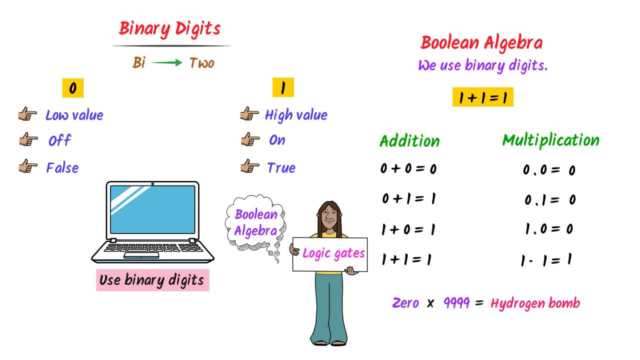 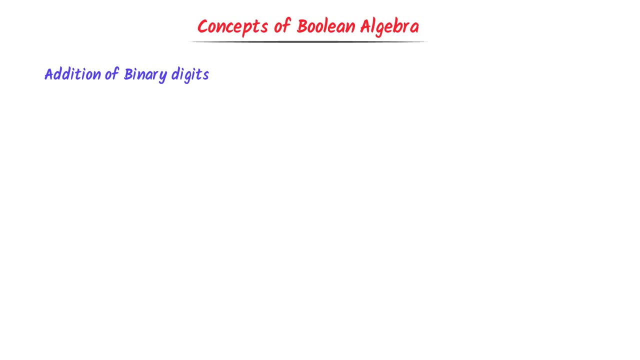 cannot learn a single concept of logic gates. Hence I will teach you some basic concepts of boolean algebra. Firstly, let me teach you addition of binary digits. Let a is equal to zero, or a is equal to one. Now a plus one is equal to one. We know that a is equal. 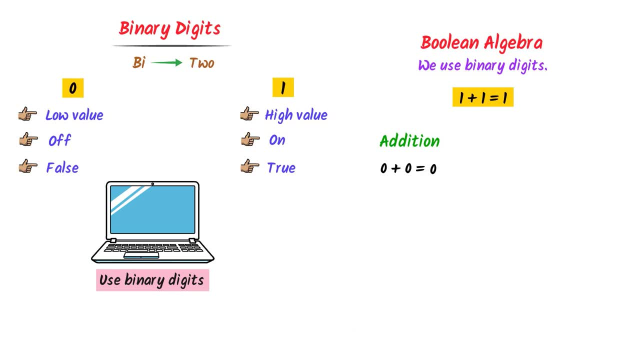 We know that zero plus zero is equal to zero. Zero plus one is equal to one. One plus zero is equal to one. One plus one is equal to two, But in boolean algebra there is no such digit like two, So one plus one is equal to one. Secondly, consider multiplication. 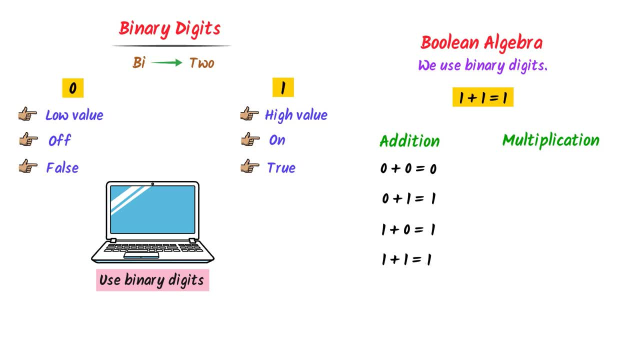 of binary digits in boolean algebra. Remember that zero and multiplication is a hydrogen bomb. It finishes everything. Let me repeat it: Zero and multiplication is a hydrogen bomb and it finishes everything. Like zero and two, zero is equal to zero. Zero and two: one. 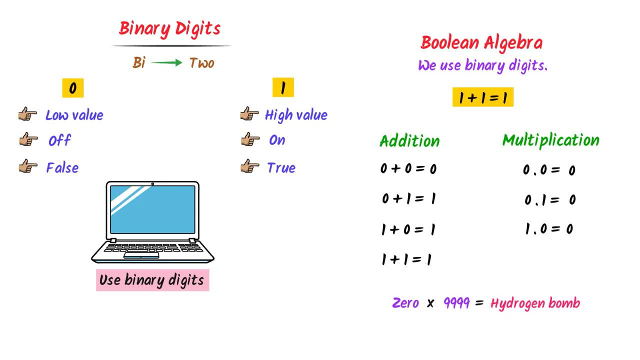 is equal to zero. One and two: zero is equal to zero. And one and two, one is equal to one. Thus, remember that in boolean algebra, all the mathematical operations are the same, except one plus one is equal to one. Now, if you want to learn the logic gates, you must learn boolean algebra. You should. 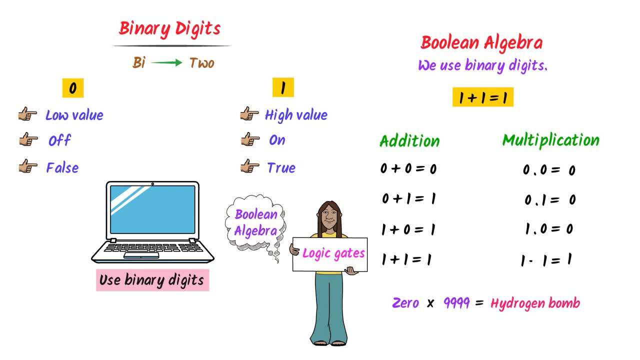 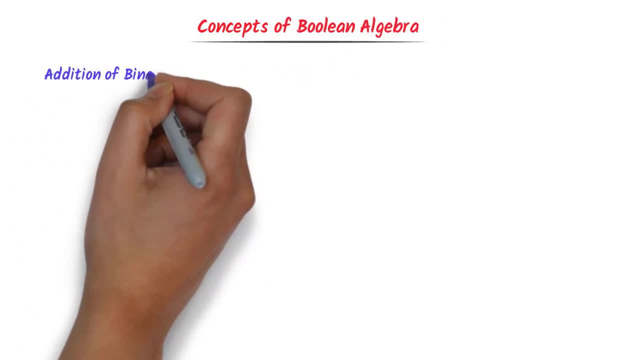 study. So 0 plus 1 is equal to 1 or 1 plus 1 is equal to 1.. Secondly, a plus 0 is equal to a. We know that a is equal to 0 or a is equal to 1.. 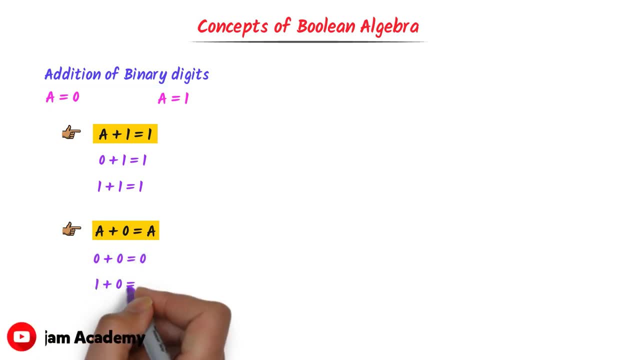 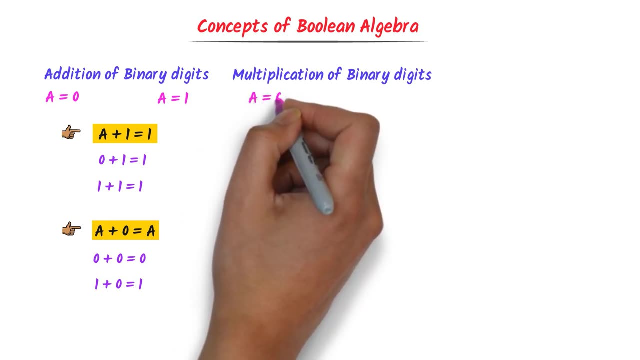 So 0 plus 0 is equal to 0, or 1 plus 0 is equal to 1.. Also, let me teach you the multiplication of binary digits. Let a equals 0 or a equals 1.. Now a into 1 is equal to 1.. 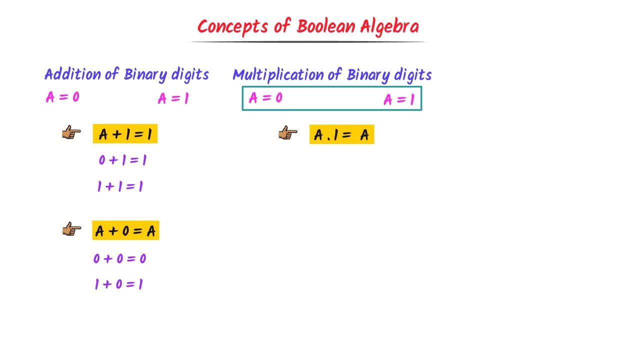 We know that a is equal to 0 or a equals 1.. So 0 into 1 is equal to 0 or 1 into 1 is equal to 1.. Secondly, a into 0 is equal to 0. We know that a equals 0 or a equals 1.. 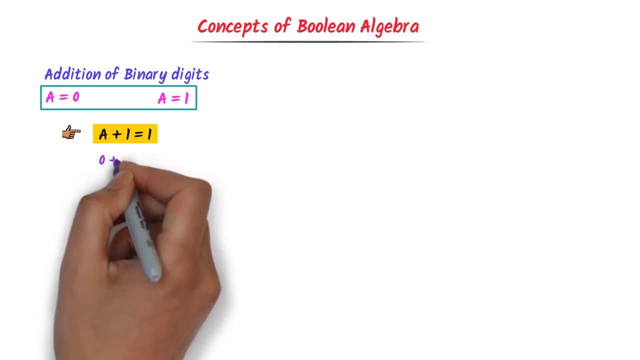 to zero or a is equal to one, So zero plus one is equal to one, or one plus one is equal to one. Secondly, a plus zero is equal to a. We know that a is equal to zero or a is equal to one, So zero plus zero is equal to zero, or one plus zero is equal to one. 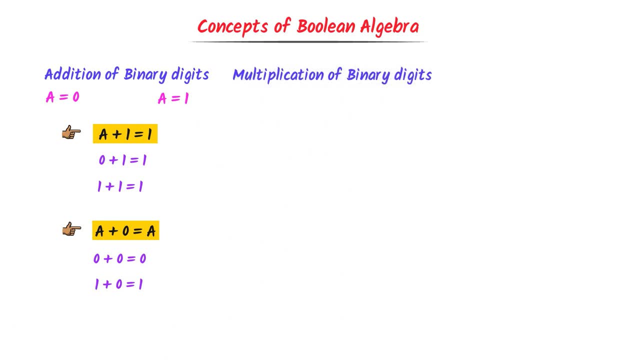 Also, let me teach you the multiplication of binary digits. Let a equal zero or a equal to one. Hence, addition of binary digits is equal to zero, and one plus zero is equal to zero. So, above, neither union is equal to zero or neither union is equal to zero. 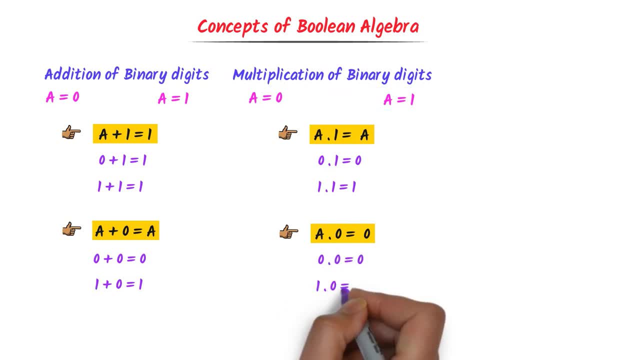 Hence, addition of binary digits is equal to zero and vice-versa. Thus, addition of binary pieces is equal to zero. Multiplication of binary digits are very simple. Now let me teach you the concept of inverse in boolean algebra. For example, consider low value. 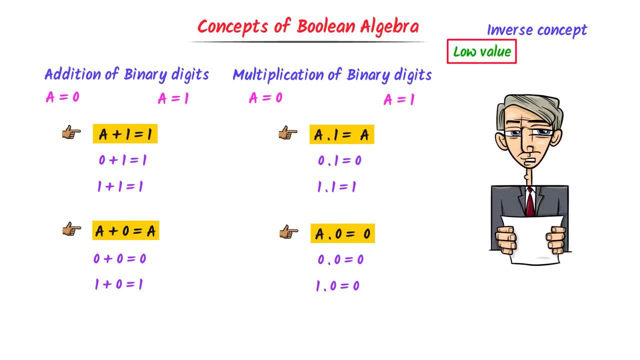 If I ask you what is its opposite value, your answer is simple: its opposite is high value. We know that 0 represents low value and 1 represents high value, So the inverse of 0 is 1 and that of 1 is 0.. 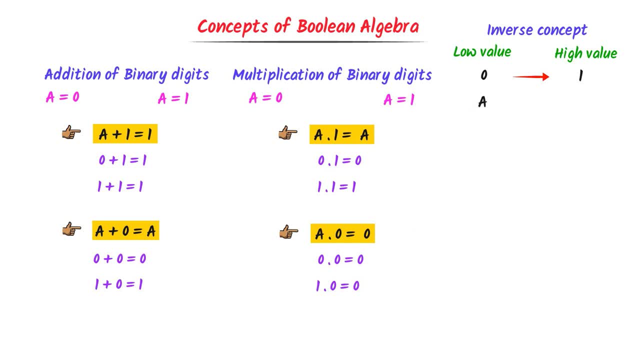 For example, if one binary digit is a, its inverse is a bar. Just remember that bar on any variable represents inverse value. Now, a plus a bar is equal to 1.. Let a equals 0.. Can you guess the value of a inverse? 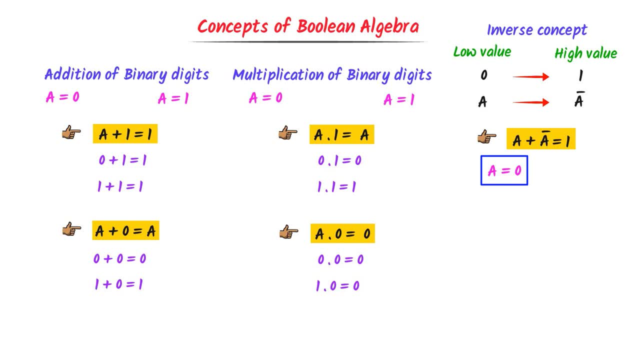 Well, a bar represents the opposite value of a. a equals 0,, a bar equals 1.. Because the opposite value of 0 is 1.. Now, 1 plus 0 is equal to 1.. Hence we say that a plus a bar equals 1.. 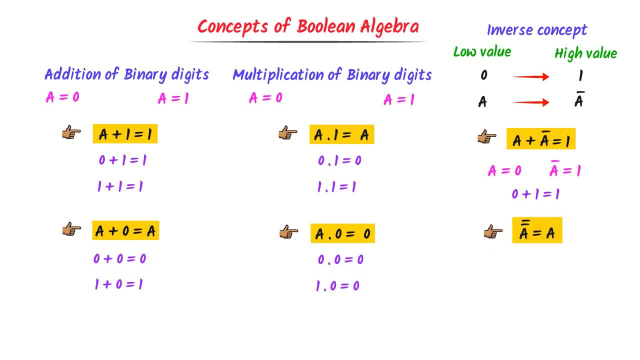 Fourthly, a double bar equals a. For example, let a equals 1.. I inverse the value of a, I get a inverse equals 0.. I again inverse the value of a, I get a double bar equals 1.. Hence the initial value of a is equal to 1.. 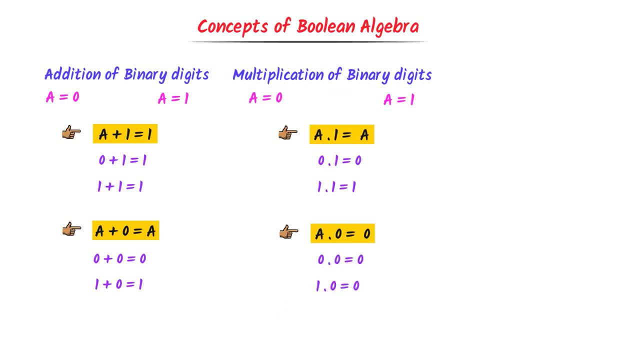 So 0 into 0 equals 0, or 1 into 0 equals 0. Hence, addition and multiplication of binary digits are very simple. Now let me teach you the concept of inverse in Boolean algebra. For example. consider low value If I ask you what is its opposite value? 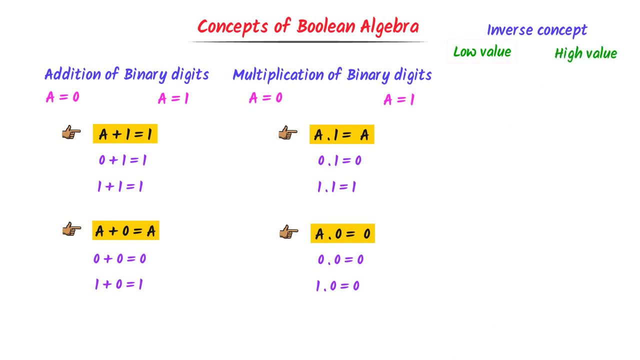 Your answer is simple. Its opposite is high value. We know that 0 represents low value and 1 represents high value. So the inverse of 0 is 1 and that of 1 is 0. For example, if one binary digit is 0, then 1 is 0. 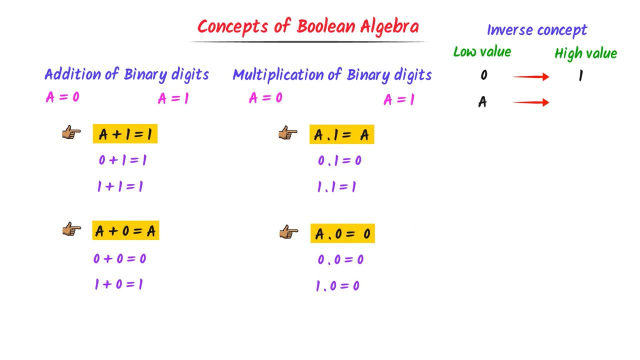 So the inverse of 0 is 1 and that of 1 is 0.. The opposite is a and its inverse is a. Thus, remember that bar on any variable represents inverse value. Now, a plus a bar is equal to 1.. Let a equals 0.. 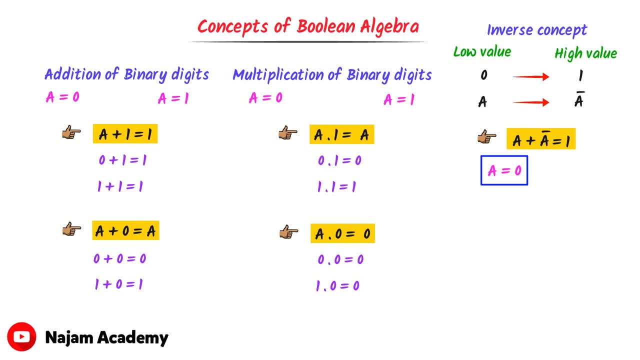 Can you guess the value of a inverse? Well, a bar represents the opposite value of a, a equals 0 and a bar equals 1, because the opposite value of 0 is 1.. And vice versa. Now, 1 plus 0 is equal to 1.. 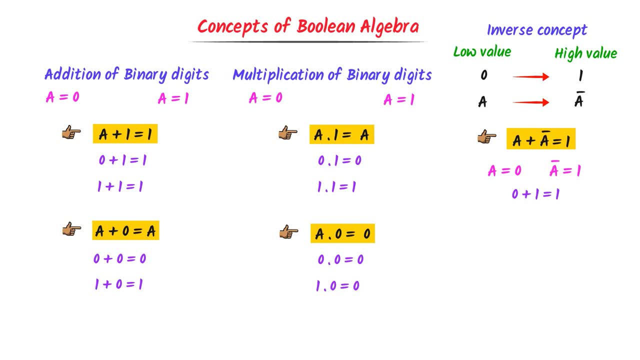 Hence we say that a plus a bar equals 1.. Fourthly, a double bar equals a. For example, let a equals 1.. I inverse the value of a. I get a inverse equals 0.. I again inverse the value of a. 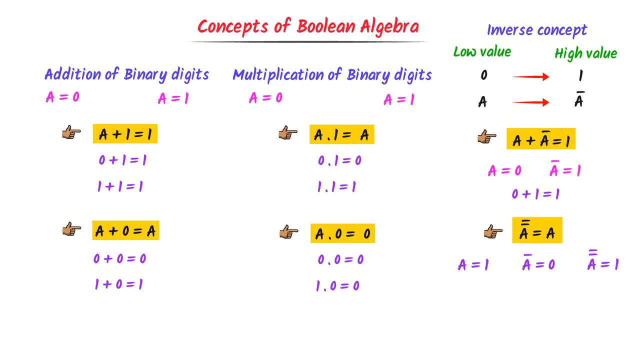 I get a double bar equals 1.. Hence the initial value of a is equal to 1. And that of a double bar is also equal to 1.. Thus we say that a double bar is equal to a. The simple trick is always: cancel the two bars. 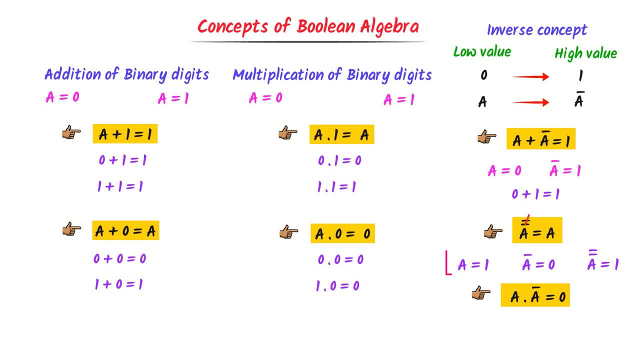 Fifthly, a dot, a bar equals 0.. Let a equals 1 and a bar becomes 0. Now 1 into 0 is equal to 0.. Thus, a into a bar equals 0.. Thus noted down all these basic concepts of Boolean. 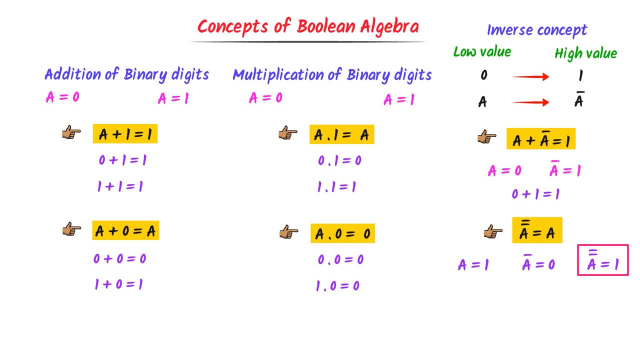 And that of a double bar is also equal to 1.. Thus we say that a double bar is equal to a. The simple trick is always: cancel the two bars. Fifthly, a dot a bar equals 0.. Let a equals 1.. 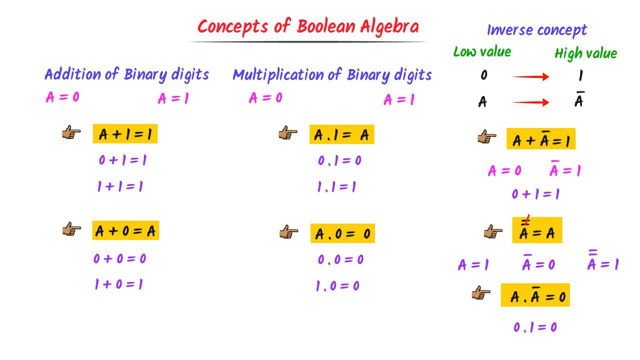 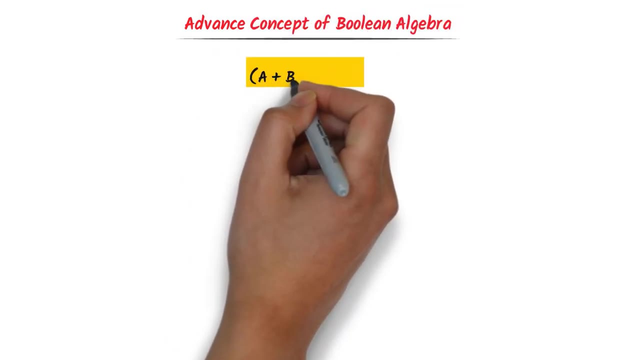 And a bar becomes 0. Now 1 into 0 is equal to 0.. Thus, a into a bar equals 0.. Thus noted down all these basic concepts of Boolean, Now I will teach you one advanced concept of Boolean Algebra: a plus b whole bar equals a bar plus b bar. 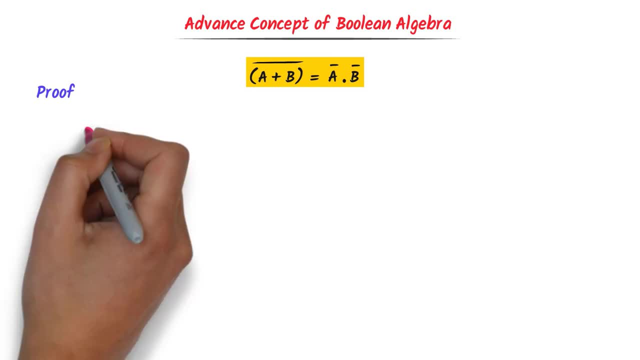 Let me also teach you its proof. Firstly, consider left hand side. At the left hand side we have a plus b, whole bar. Now consider values of a and b. Let a equals 1 and b equals 0. Because here we can use only these two digits. 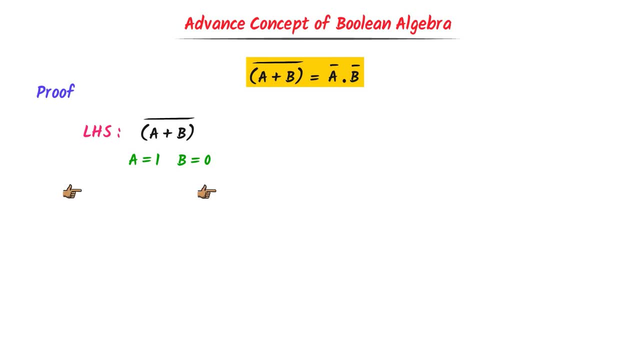 I will solve this question in two steps. In the first step, I will find a plus b. In the second step, I will find inverse of a plus b. Now, in the first step, a plus b is the value of a is 1 and that of b is 0.. 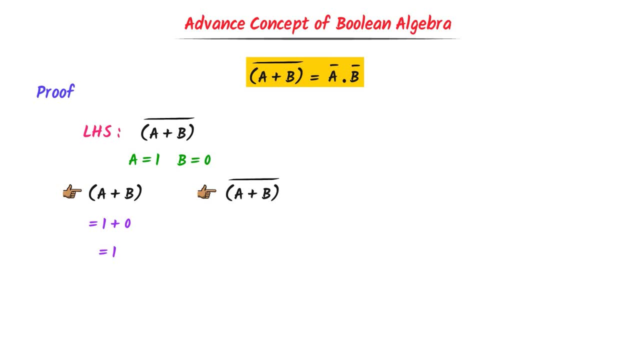 1 plus 0. I get 1.. Hence the value of a plus b is equal to 1.. In the second step we have to inverse the value of a plus b. We know that a plus b is equal to 1 and its inverse is 0.. 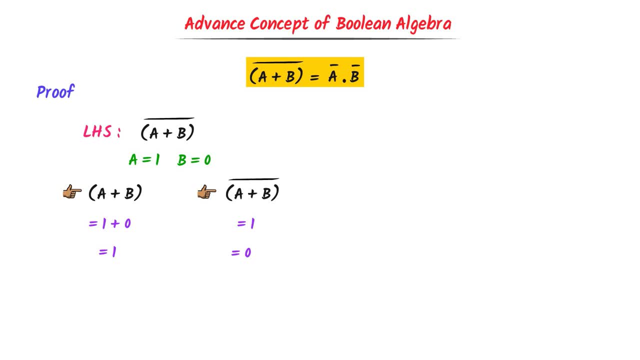 Thus, at the left hand side, a plus b, whole inverse, is equal to 0. Let, this is equation number 1.. Now at the right hand side we have a bar, dot b bar. We know that a equals 1 and b equals 0.. 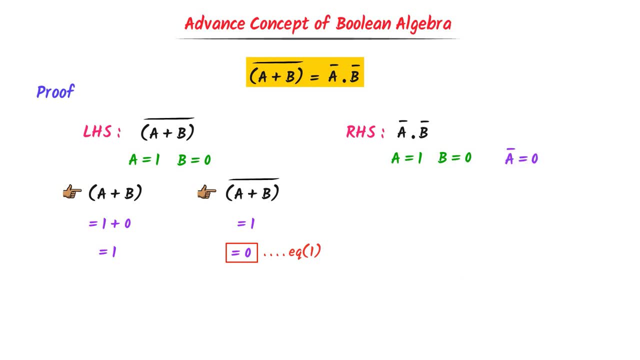 Now the value of inverse a is equal to 0 and the value of inverse b bar is equal to 1.. According to the given statement, we have to multiply a inverse and b inverse. I write 0.1.. I get 0.. 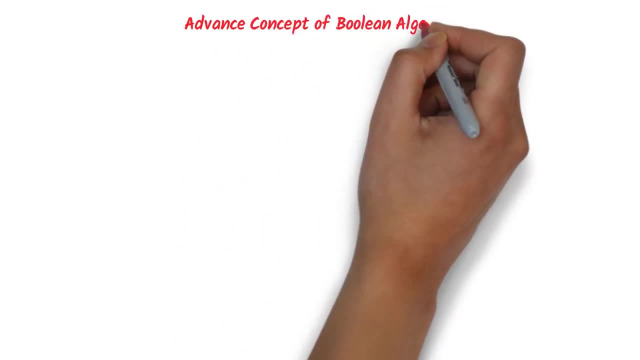 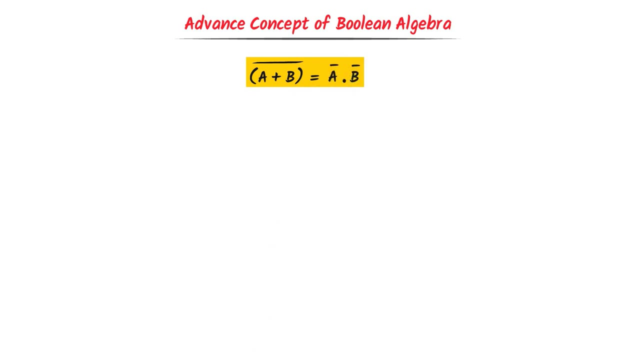 I'll show you how to do it. Now I will teach you one advanced concept of Boolean Algebra: a plus b whole bar equals a bar plus b bar. Let me also teach you its proof. Firstly, consider left-hand side. At the left-hand side we have a plus b whole bar. 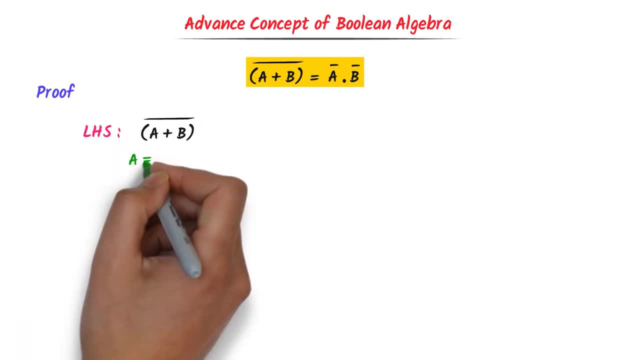 Now consider values of a and b. Let a equals 1 and b equals 0. Because here we can use only these two digits. I will solve this question in two steps. In the first step, I will find a plus b. 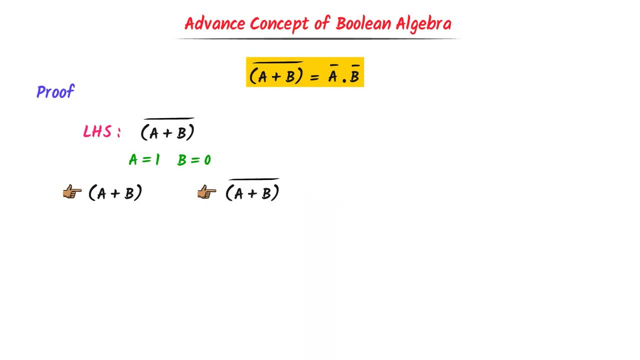 In the second step I will find inverse of a plus b. Now in the first step, a plus b is the value of a is 1 and that of b is 0.. 1 plus 0. I get 1.. 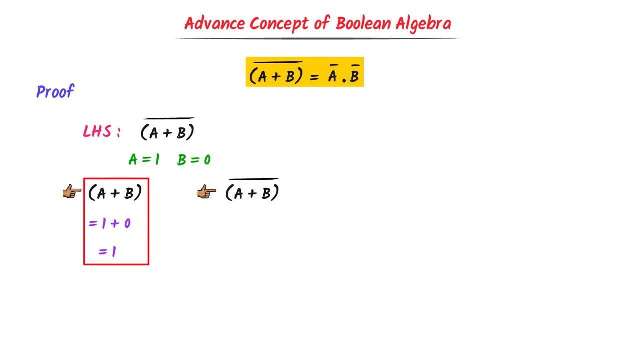 Hence the value of a plus b is equal to 1.. In the second step we have to inverse the value of a plus b. We know that a plus b equals 1.. A plus b is equal to 1 and its inverse is 0.. 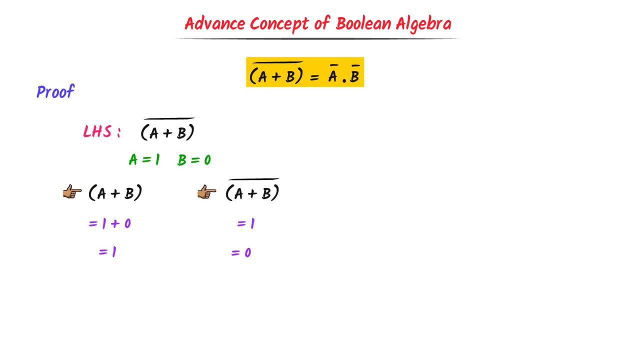 Thus, at the left-hand side, a plus b, whole inverse, is equal to 0.. Let, this is equation number 1.. Now at the right-hand side we have a bar, dot b bar. We know that a equals 1 and b equals 0.. 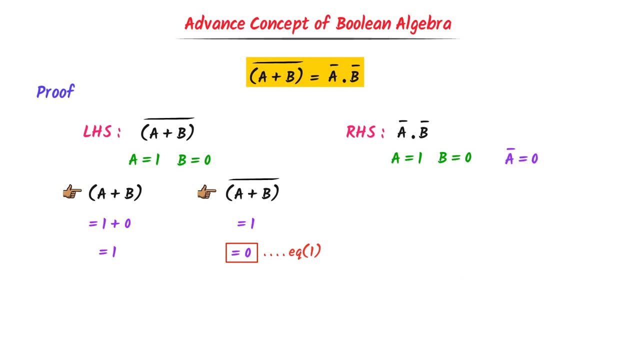 Now the value of inverse a is equal to 0 and the value of inverse b bar is equal to 1.. In the third step we have to multiply a inverse and b inverse. I write 0.1.. I get 0.. 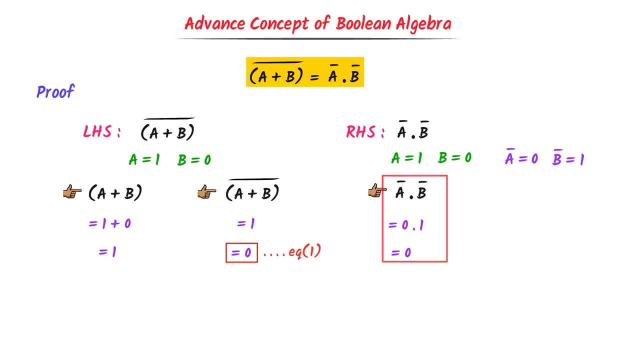 Thus the value of a bar dot b bar equals 0.. Let, this is equation number 2.. We can see that equation number 1, a plus b whole bar equals 0, and equation number 2, a bar, dot b bar is also equal to 0. 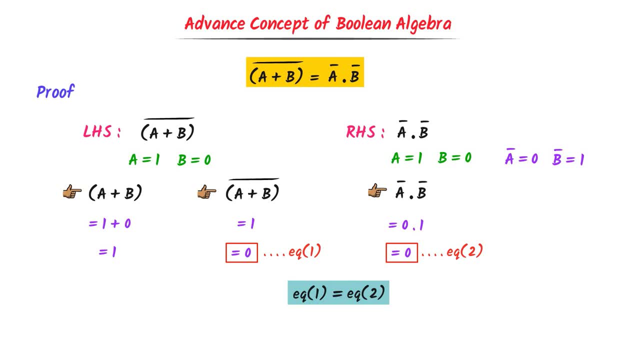 Hence, equation number 1 is equal to equation number 2.. Therefore, this is equation number 1.. We write 0.. We write 0.. We write a bar dot b bar. This is equation number 1.. Then let this equation number 1 be 0.. 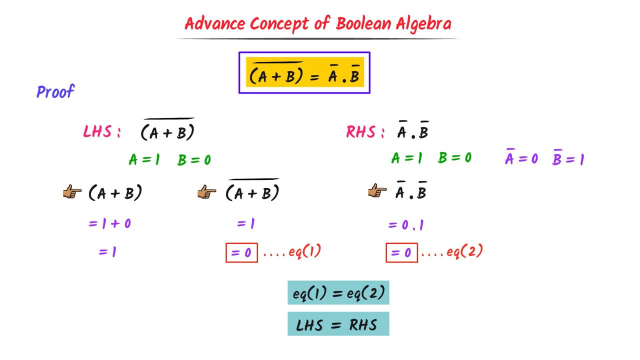 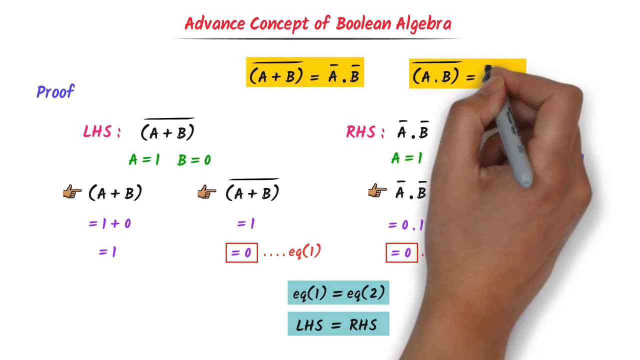 And then let's write 0. What is this equation number 1?? Well, this equation number 1 is equal to 0. So you can see that 0 is equal to a bar dot b bar. Similarly, a dot b whole bar is equal to a bar plus b bar. 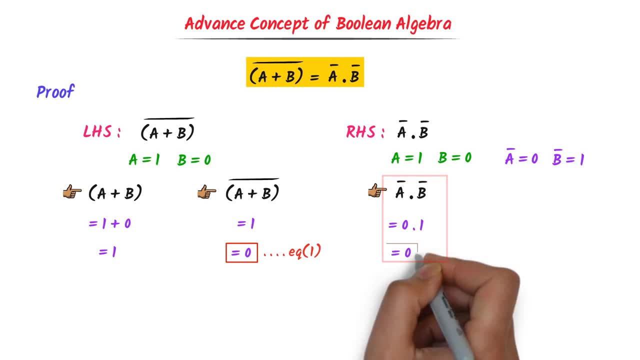 Thus the value of a bar dot b bar equals 0.. Let, this is equation number 2.. We can see that equation number 1, a plus b whole bar equals 0, and equation number 2, a bar, dot b bar is also equal to 0. 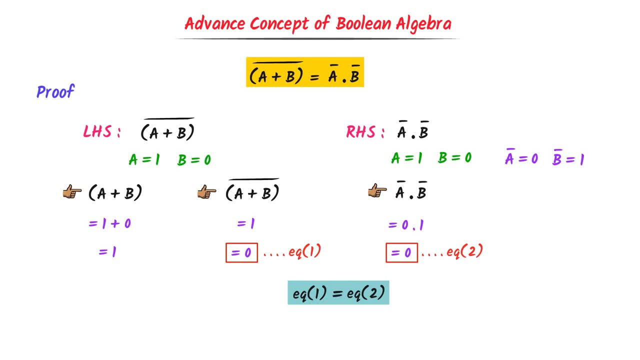 Hence equation number 1 is equal to 0.. Hence equation number 2, a bar dot b bar is also equal to 0. Hence equation number 1 is equal to 0.. Hence equation number 2, a plus b, whole bar, equals a bar dot b bar. 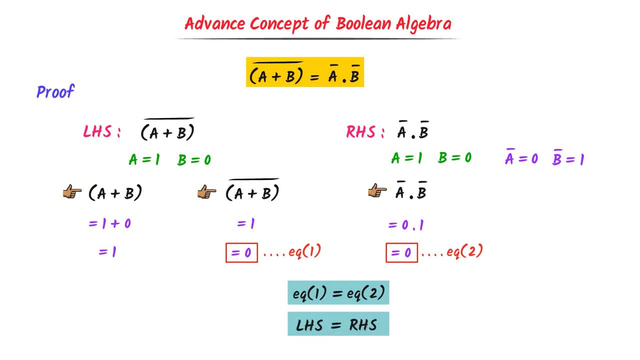 Now suppose we write a plus b whole bar equals 0. they are equal to 0.. Let us write: a plus b whole bar equals a bar dot b bar. Similarly, a dot b whole bar equals a bar plus b bar. Now I will teach you my personal and super easy trick to remember these two equations. 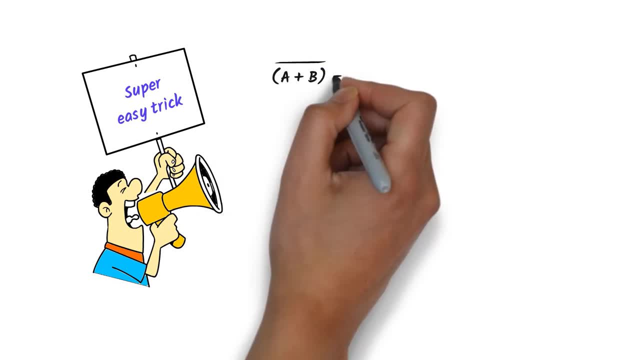 Let I write a plus b whole bar equals a bar, dot b bar and ab whole bar. I always write a bar b bar, a bar b bar. Secondly, if there is plus, I convert it to dot. If there is dot, I convert it to plus. This is the super fast, easy trick. 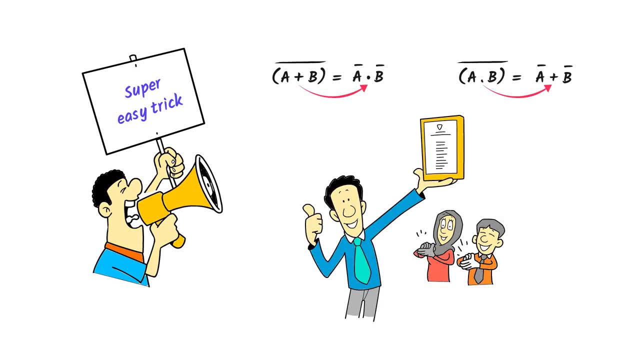 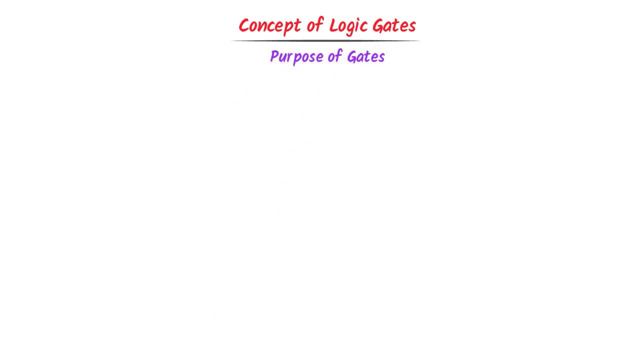 to remember these two equations. Now it is time to teach you the easy concepts of logic gates. Firstly, let understand the basic purpose of a gate. Consider this open door and this closed door. In case of open door, you are allowed to pass through. In case of closed door, you 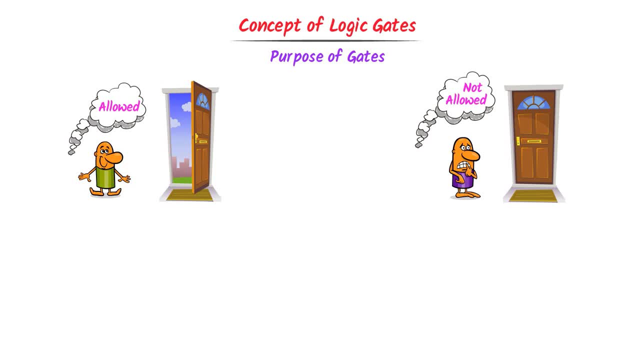 are not allowed to pass through. Similarly, consider these logic gates. Logic gates either do not allow electrical signal to pass through, or logic gates allow electrical signal to pass through. I mean these two same gates. They are not connected. They are not connected. 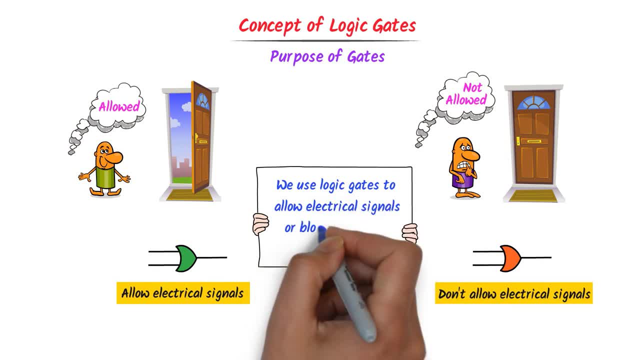 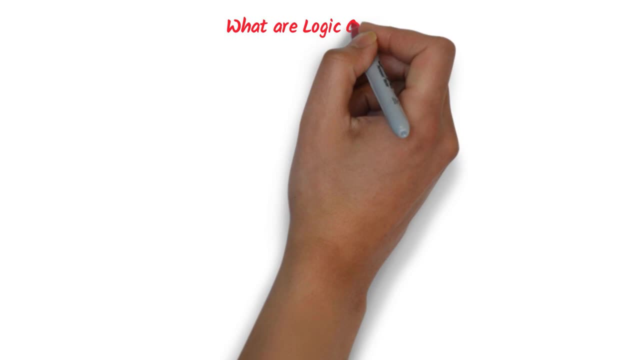 we use logic gates in order to allow our block electrical signals, or digital signals, to enter into the circuit. Thus, remember that we use logic gates to on and off any digital circuit. Now, what are logic gates? Well, consider this logic gate. We give two inputs to any logic gate. 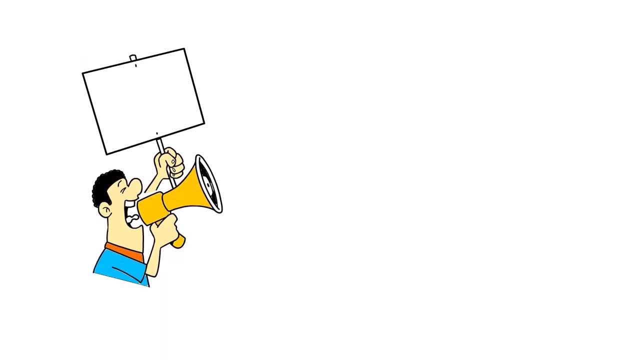 Now I will teach you my personal and super easy trick to remember these two equations. Let us write a dot b whole bar and a dot b whole bar. So what is our solution for this? Let's know, bar, I always write a bar b bar, a bar b bar. Secondly, if there is plus, I convert it to 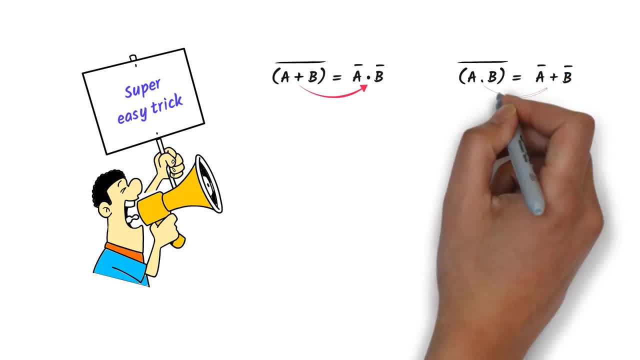 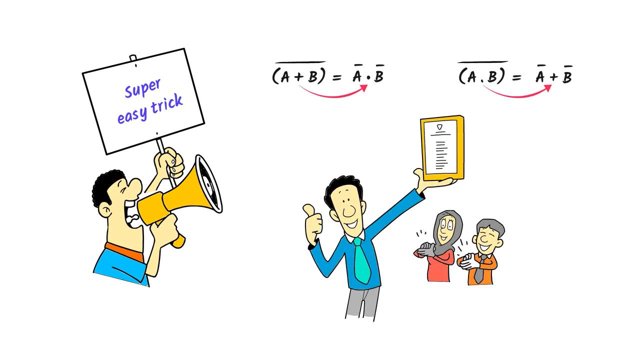 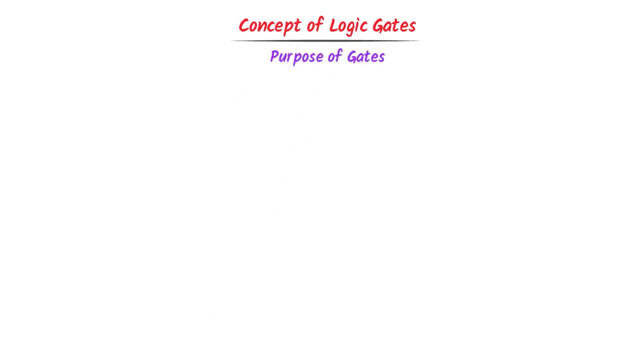 dot. If there is dot, I convert it to plus. This is the super fast, easy trick to remember these two equations. Now it is time to teach you the easy concepts of logic gates. Firstly, let understand the basic purpose of a gate. Consider this open door and this closed door. 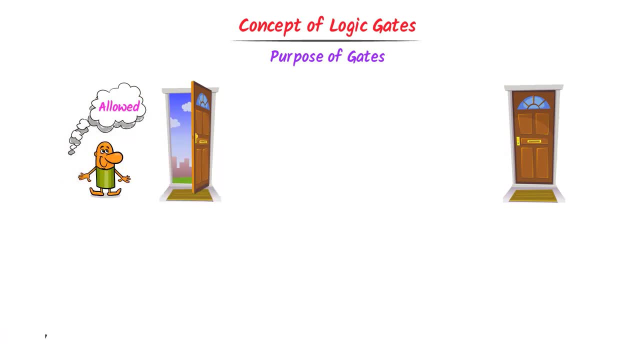 In case of open door, you are allowed to pass through. In case of closed door, you are not allowed to pass through. Similarly, consider these logic gates. Logic gates either do not allow electrical signal to pass through, or logic gates allow electrical signal to pass through. 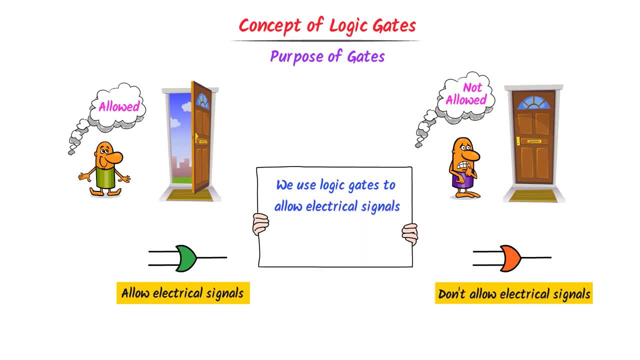 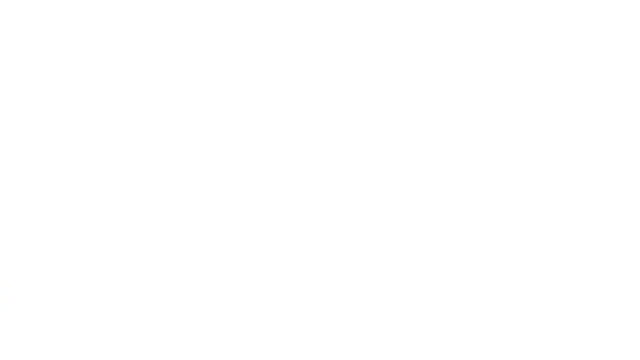 I mean we use logic gates to pass through. Wo will we do this? Before we, before we begin the law, you must have some logical inputs in your logic system. in order to do so, you have to take a number of log1 to log2. 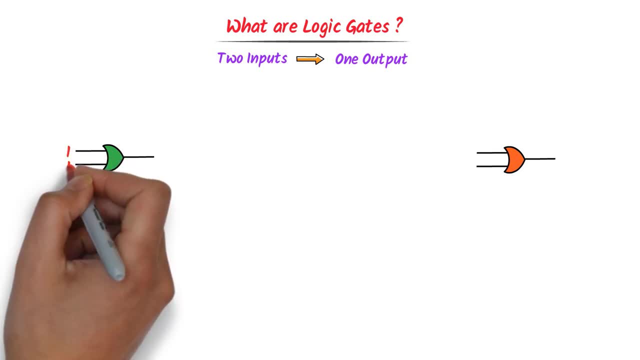 You must havecoin groups to take aent- How you do it- to apply the изв. You may also take win to take a Morgan min to this logic gate. We know that 1 represent on This logic gate will give us 1 as output. 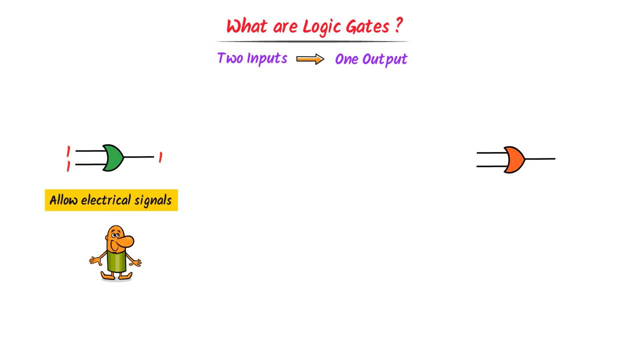 So it allow the digital signal to pass through. Secondly, consider this logic gate. I give two inputs to it: 0 and 0. We know that 0 represents off. This logic gate will give us 0 as output, So it does not allow digital signal to pass through. Thus we give two inputs to a logic. 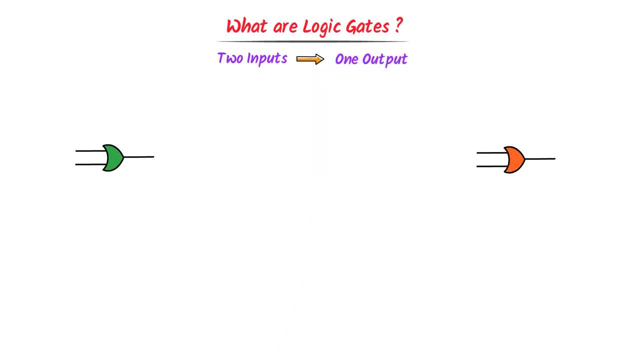 and we get only one output. For example, I give 1 and 1 as inputs to this logic gate. We know that 1, represent on This logic gate, will give us 1 as output, So it allow the digital signal to pass. 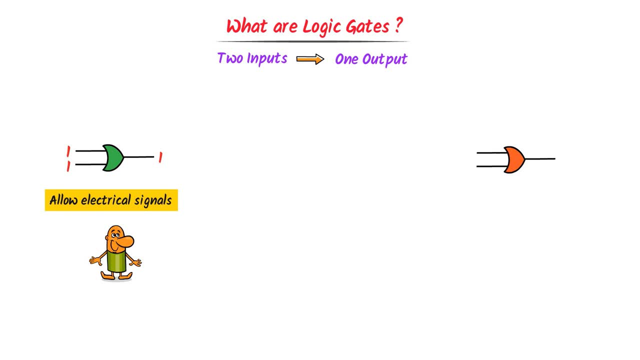 through. Secondly, consider this logic gate. I give two inputs to it: 0 and 0.. We know that 0 represents off. This logic gate will give us 0 as output, So it does not allow digital signal to pass through. 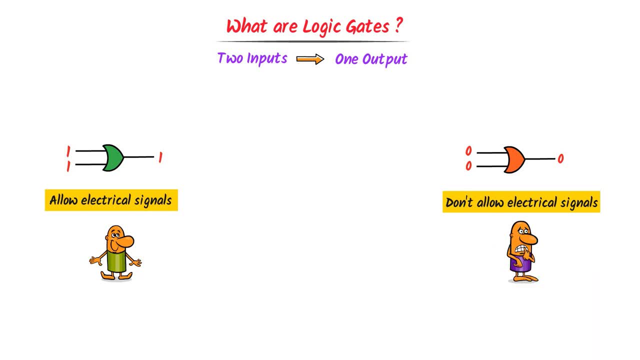 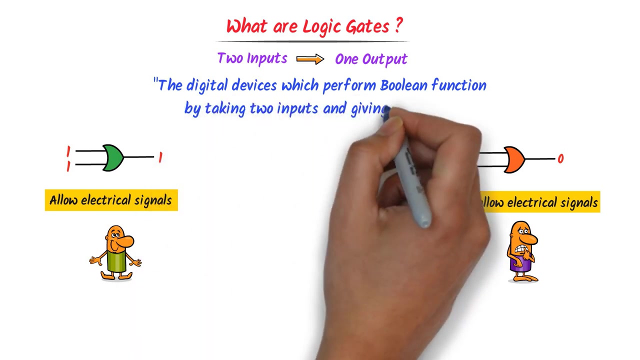 Thus, we give two inputs to a logic gate, It performs a boolean function and gives us an output. Therefore, we define logic gates as the digital devices which perform boolean function by taking two inputs and giving an output. Let me repeat it: The 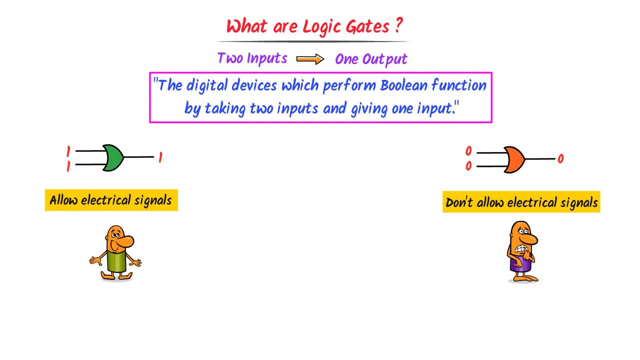 digital devices which perform boolean function by taking two inputs and giving an output. Remember that logic gates work on the principles of boolean algebra. Secondly, logic gates are made up of diodes and transistors. Thus, remember that, with the help of boolean algebra, logic gates, 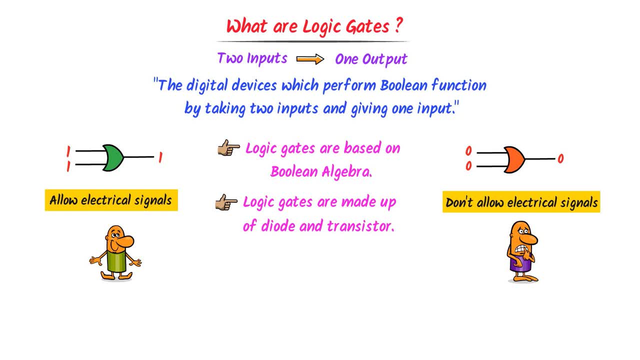 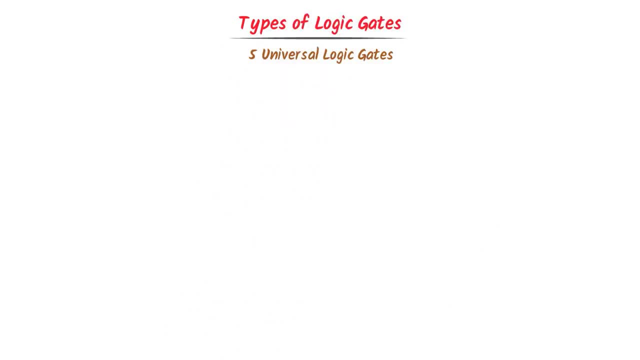 either allow or block signals in order to enter into the circuit. Now, what are the types of basic logic gates? Well, there are five universal logic gates. Firstly, we'll learn three logic gates like OR AND NOT. In case of OR gate, I halfy cut the o, I draw it here and I curve. 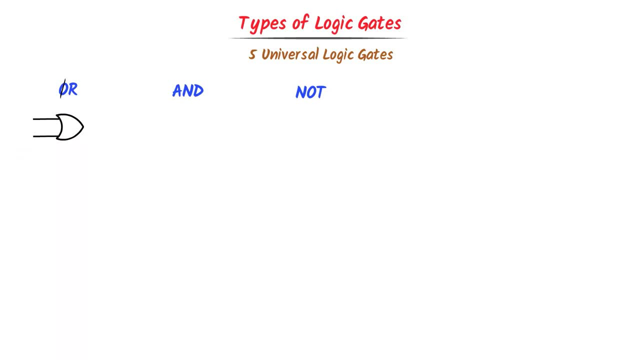 this side, We always give two inputs to the logic gate, like A and B. Use these inputs to give us an output. y. At my practice with logic gateway, I was thinking of the logic gate in this Ravelening equation. However, we'll study the logic gate in details in the next part. Let get started. Thank you for watching and Don't get confused. you can find it at my page. Thank you for watching and Don't forget to subscribe. Thank you for watching and Don't forget to subscribe to my page and bill us a video daily, lowered to 0, so that we can get this tutorial. tutorial. 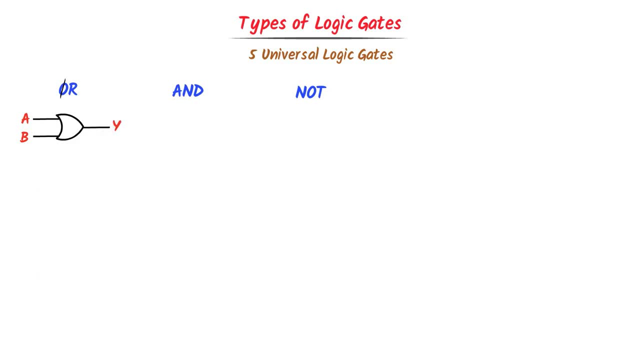 At my page we have� n inputs toCLavy wva1. us. an output Y. Now the question is how this OR gate process these two endports A, B. Well, OR gate add these two endports A and B. So I write: output: Y is equal to A plus B. Now consider this truth. 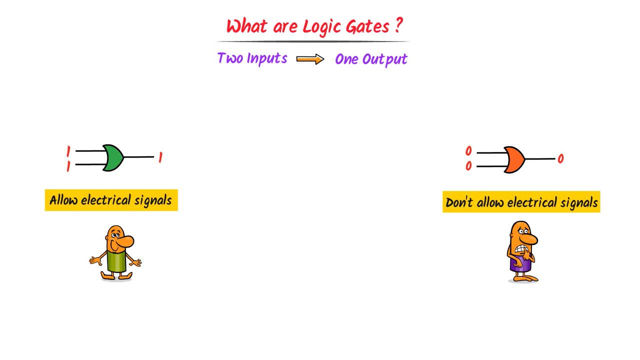 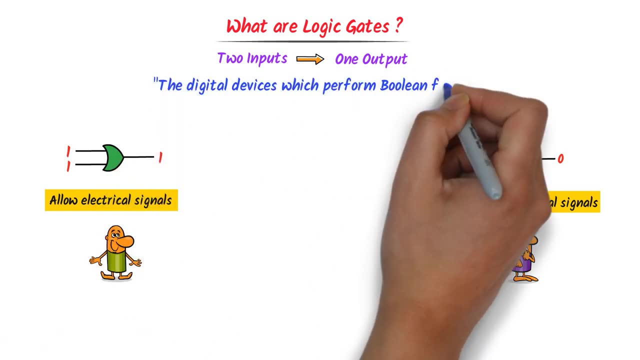 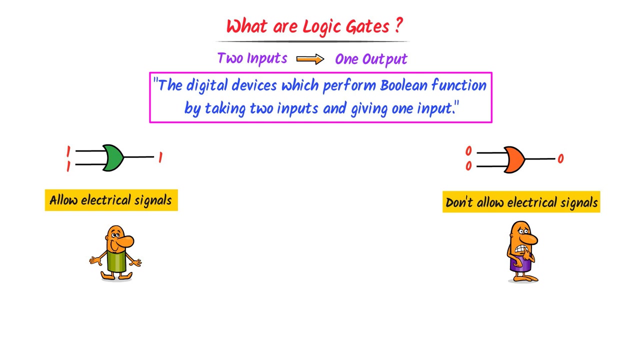 gate. It performs a boolean function and give us an output. Therefore, we define logic gates as the digital devices which perform boolean function by taking two inputs and giving an output. Let me repeat it: The digital devices which performs boolean function by taking two inputs and giving an output. Remember that logic gates work on the principles of: 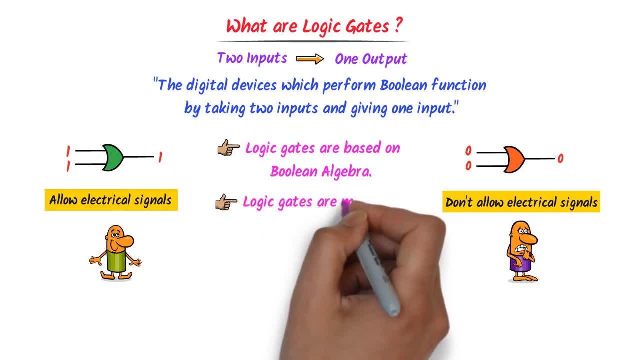 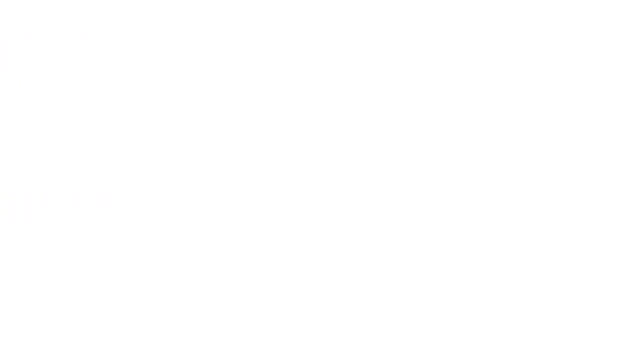 boolean algebra. Secondly, logic gates are made up of diodes and transistors. Thus, remember that, with the help of boolean algebra, logic gates either allow or block signals in order to enter into the circuit. Now, what are the types of basic logic gates? Well, there are. 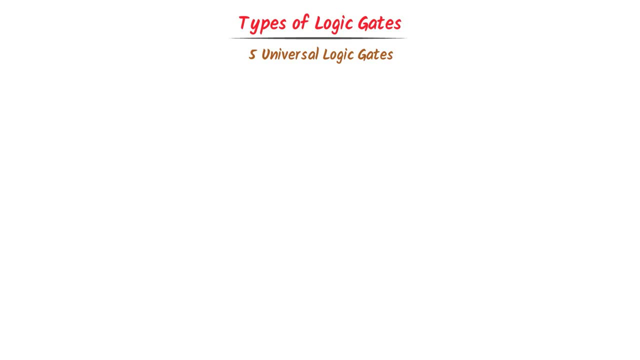 5 universal logic gates. Firstly, we will learn three logic gates like OR and NOT. In case of OR gate. I half ly cut the O, I draw it here and I curve this side. We always give two inputs to the logic gate, like A and B. Use these inputs to give us an output Y. Now the question is how? this 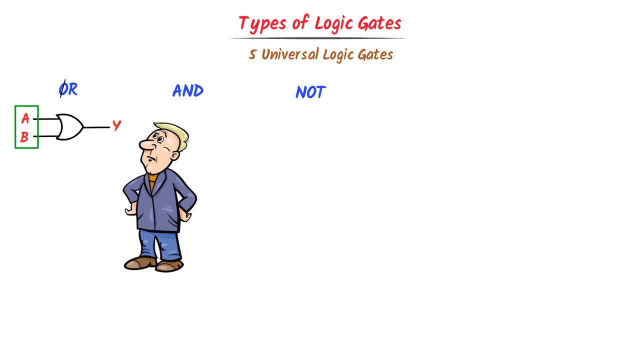 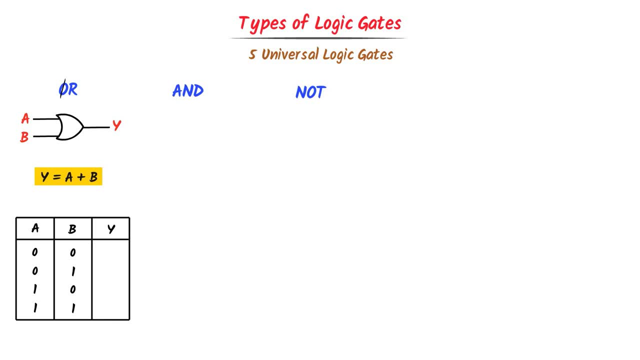 table. We know that the possible value of AB is either 0, 0,, 0, 1,, 1, 0 or 1, 1.. What about the value of Y? Well, OR gate, always sum up the value: 0 plus 0 is equal to 0.. 0 plus 1 is equal to 1.. 1 plus 0. 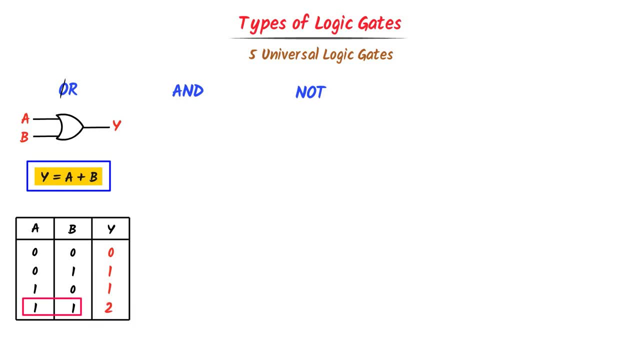 is equal to 1.. 1 plus 1 is equal to 2.. But in Boolean algebra there is no such digit like 2.. So 1 plus 1 is equal to 1.. Thus this is the truth. table of OR gate. Secondly, in case of AND gate. 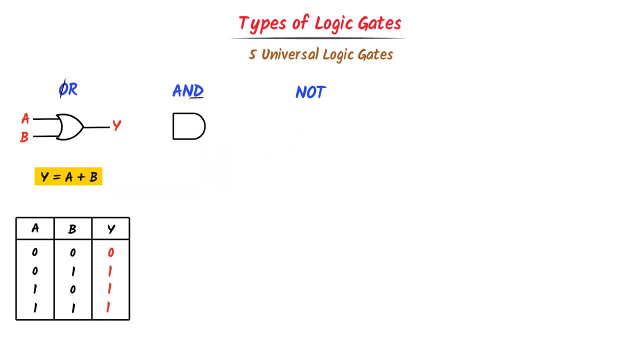 I take this D, I write it here. I give two endports, A and B. It give us an output Y. Now how this AND gate process these two endports A and B. Well, in case of AND gate, this D reminds me dot, I mean Y is. 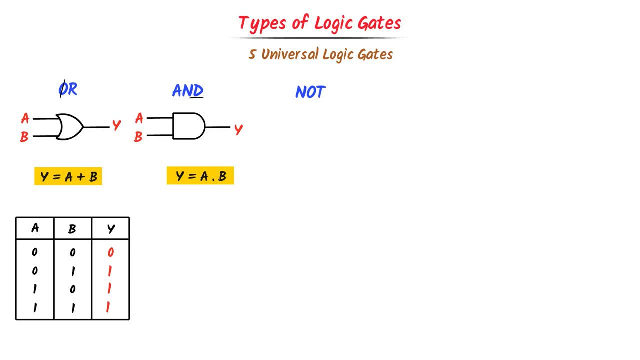 equal to A dot B. So AND gate multiply A and B to give us an output Y. Now consider this truth table along with the possible value. What about the value of Y? Well, AND gates multiply A and B are: AND gate multiply endports. 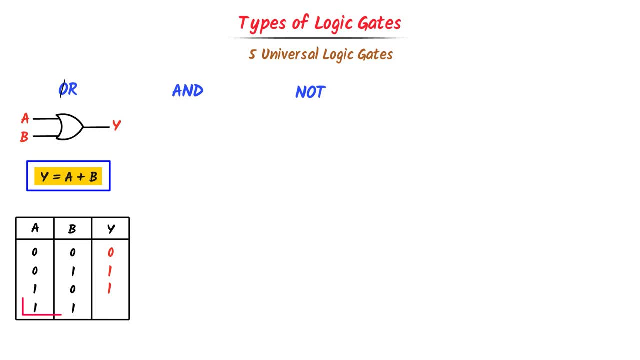 digit like 2.. So 1 plus 1 is equal to 1.. Thus this is the truth. table of OR gate. Secondly, in case of AND gate, I take this D, I write it here. I give two inputs: A and. 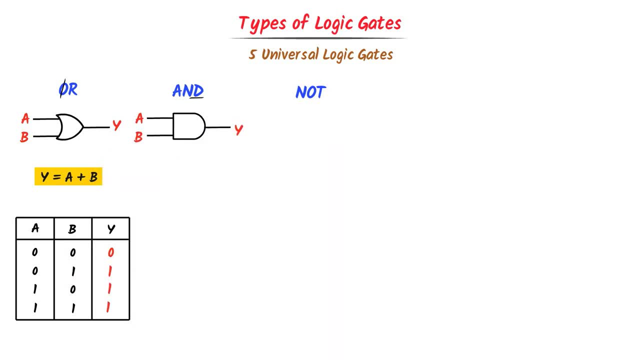 B, It give us an output Y. Now how this AND gate process these two inputs, A and B? Well, in case of AND gate, this D reminds me dot. I mean Y is equal to A, dot B. So AND gate multiply A and B to give us: 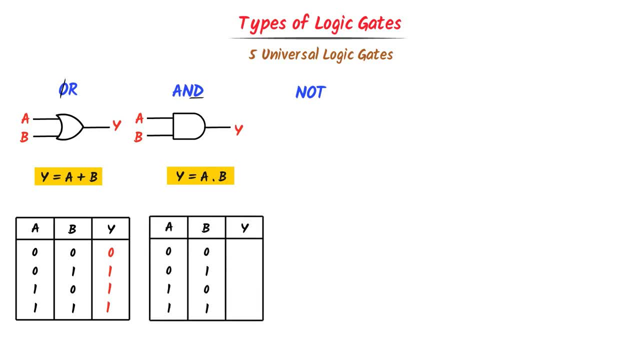 an output: Y. Now consider this truth table along with the possible values of A and B. What about the value of Y? Well, AND gates: multiply A and B. A AND gate multiply A and B are: AND gate multiply AND ports: 0 into 0 is equal to 0.. 0 into 1 equals 0.. 1 into 0 equals 0.. 1 into 1 equals 1.. Thus, 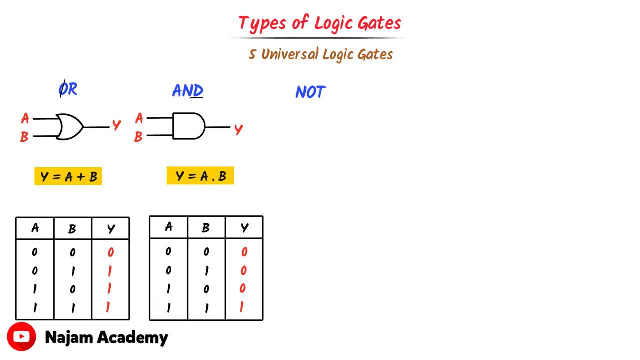 this is the truth. table of AND gate. Thirdly, in case of NOT gate, I halfly cut the AND and I write it here like this: Also, I select this O and I write it here. I give one AND put a to NOT gate. Remember that NOT gate inverse the value of input, So its output. 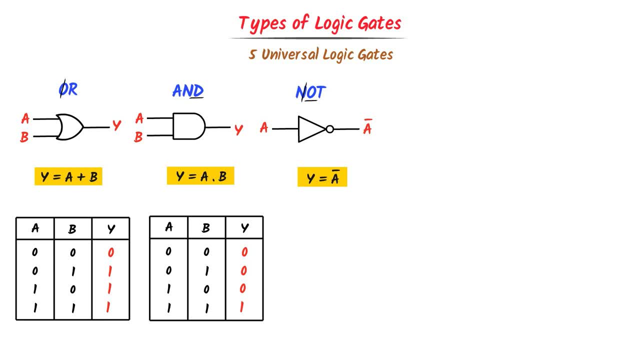 is a bar, or y equals a bar, For example. consider this truth table: The possible values of a is 1 and 0.. What about the value of y? Well, just inverse the value of a. The inverse of 1 is 0 and that of 0 is 1.. Hence, this is the truth table of, NOT gate. 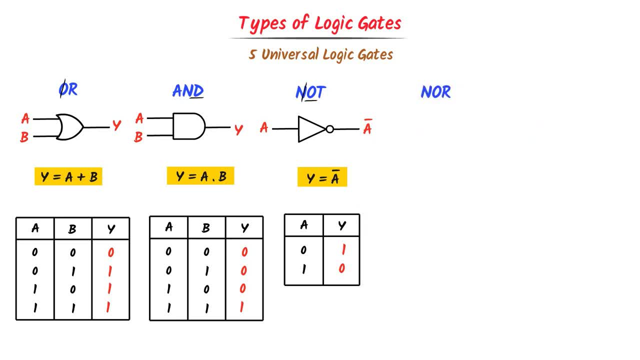 Now the fourth gate is NOR gate. We take NOT gate and OR gate to form NOR gate Here. I draw OR gate and I just put only small circle in front of it. This is the NOR gate. Now listen carefully. The OR gate will add the inputs a plus b and the NOR gate will inverse. 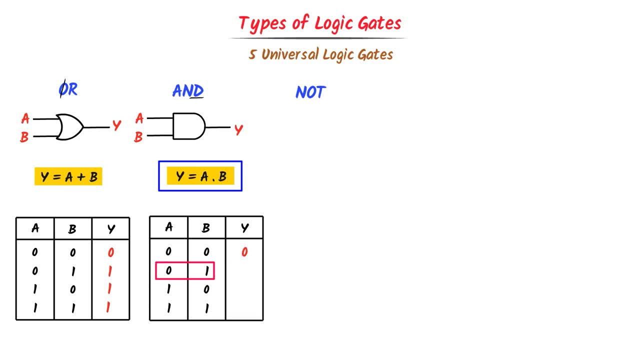 0 into 0 is equal to 0.. 0 into 1 equals 0.. 1 into 0 equals 0.. 1 into 1 equals 1.. Thus, this is the truth. table of AND gate. Thirdly, in case of NOT gate, I halfly cut the AND and I write it here like this: 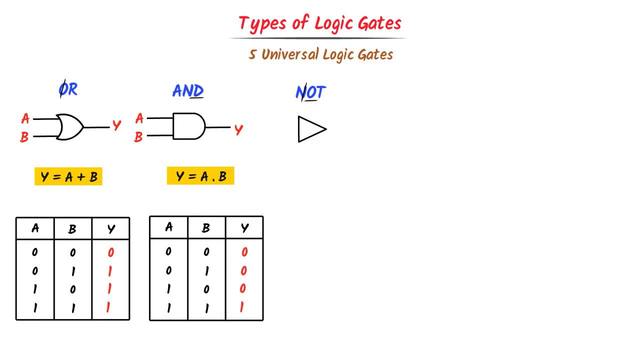 Also, I select this O and I write it here. I give one endport, A, to NOT gate. Remember that, NOT gate. inverse the value of endport, So its output is A bar. Our Y equals A bar. For example, consider this truth table: The possible values of A is 1 and 0. What about the value of Y? Well, just inverse. 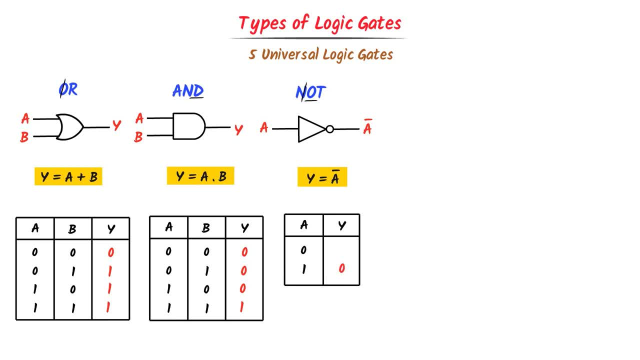 value of a, The inverse of 1 is 0 and that of 0 is 1.. Hence, this is the truth. table of NOT gate. Now the fourth gate is NOR gate. We take NOT gate and OR gate to form NOR gate. Here I draw OR gate. 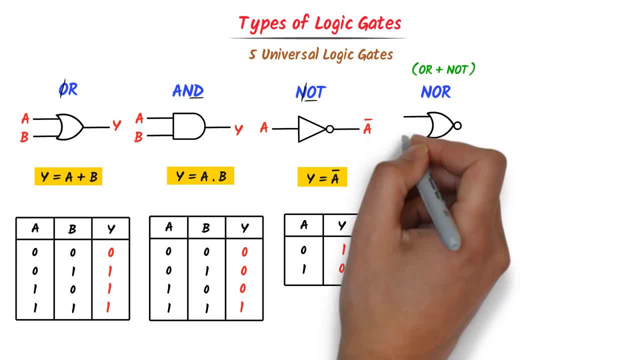 and I just put only small circle in front of it. This is the NOR gate. Now listen carefully. The OR gate will add the inputs a plus b and the NOR gate will inverse it. Let me repeat it: The OR gate will add the inputs a and b and the NOT gate will inverse it. So I write OR gate y. 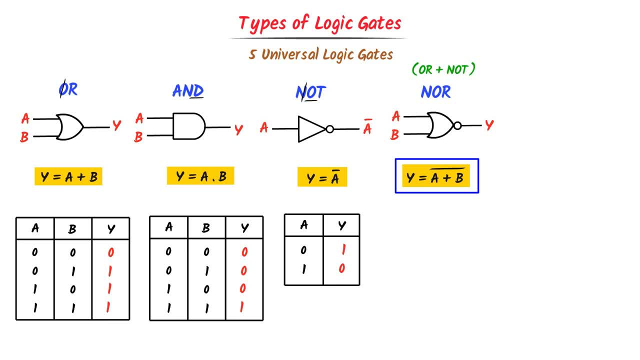 is equal to a plus b, then I put bar on it, because NOT gate inverse it. What about its truth table? Well, consider these possible values of a and b Now, OR gate will add them: 0 plus 0 is equal to 0,. 0 plus 1 is equal to 1,. 1 plus 0 is equal to 1,. 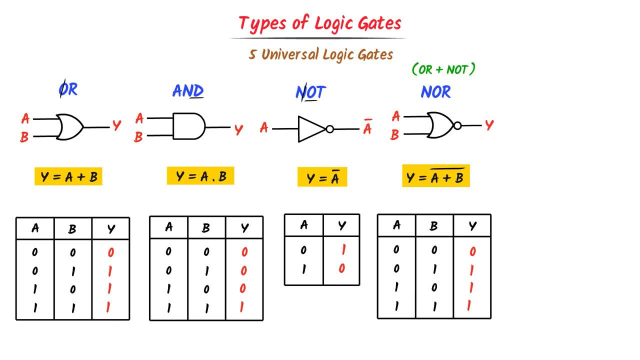 1 plus 1 is equal to 1.. Also, we know that the NOT gate will inverse them. Inverse of 0 is 1 and that of 1 is 0. I write 0 0, 0. Thus this is the truth. table of NOR gate. 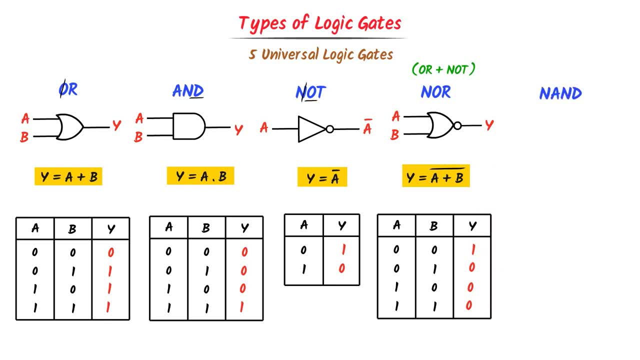 The last and the fifth gate is NAND gate. We take NOR gate and AND gate to form NAND gate. Here I draw AND gate and I put only small circle in front of it. This is the NAND gate. Now listen carefully. The AND gate will multiply the inputs. a. 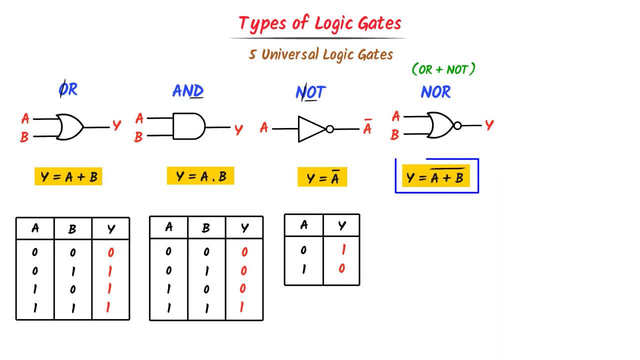 it. Let me repeat it: The OR gate will add the inputs a and b and the NOT gate will inverse it. So I write: OR gate y is equal to a plus b. Then I put bar on it because NOT gate inverse it. What about its truth table? Well, consider these possible values of a and b. 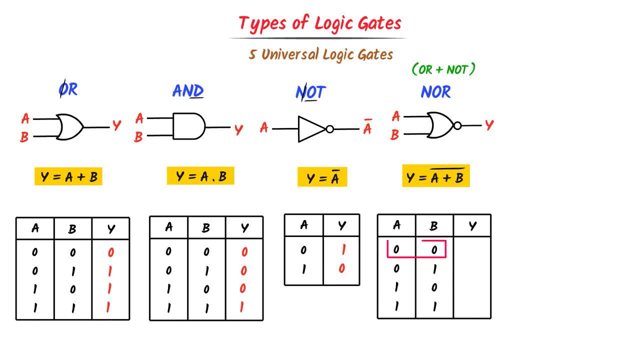 Now OR gate will add them: 0 plus 0 is equal to 0.. 0 plus 1 is equal to 1.. 1 plus 0 is equal to 1.. 1 plus 1 is equal to 1.. Also, we know. 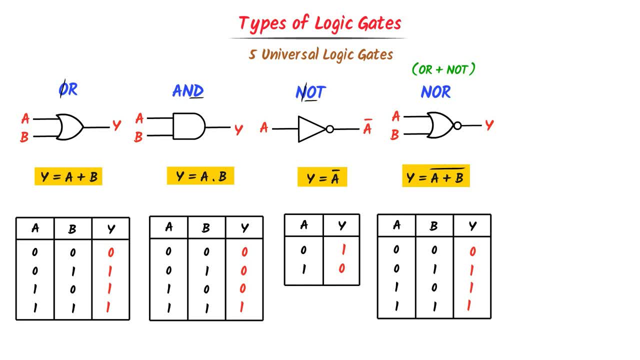 that the NOT gate will inverse them. Inverse of 0 is 1 and that of 1 is 0. I write 0, 0, 0. Thus this is the truth. table of NOR gate. The last and the fifth gate is NAND gate. We take NOT gate and AND gate to form NAND. 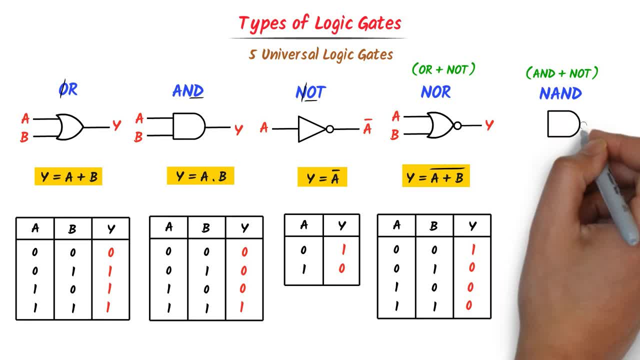 gate. I draw AND gate and I put only small circle in front of it. This is the NAND gate. Now listen carefully. The AND gate will multiply the inputs a and b and the NOT gate will inverse it. Let me repeat it: The AND gate will multiply the inputs a, b and the NOT gate will inverse. 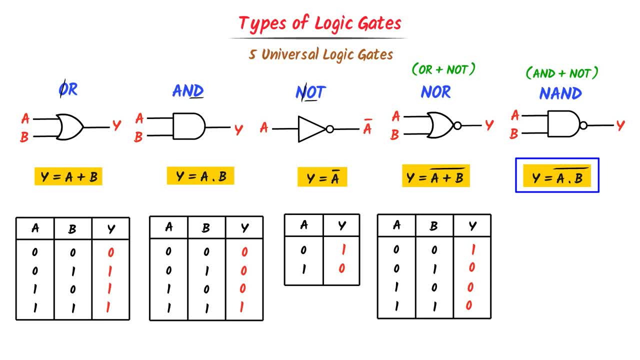 it. So I write: AND gate y is equal to a dot b. Then I put bar on it because NOT gate will inverse it. What about its truth table? Well, consider these possible values of a, b Now, AND gate will multiply them: 0 into 0 is equal to 0.. 0 into 1 is equal to 0.. 1 into 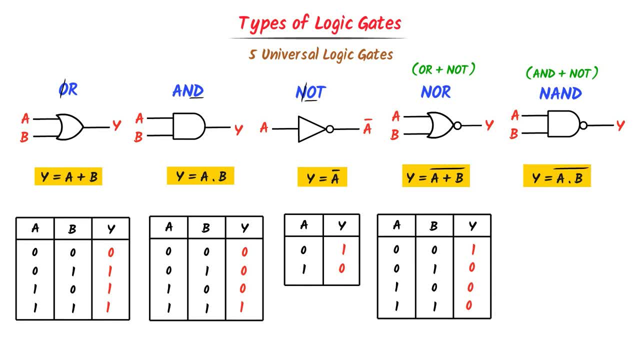 and b and the NOT gate will inverse it. Let me repeat it: The AND gate will multiply the inputs a, b and the NOT gate will inverse it. So I write: AND gate y equals a dot b. then I put bar on it because NOT gate will inverse it. 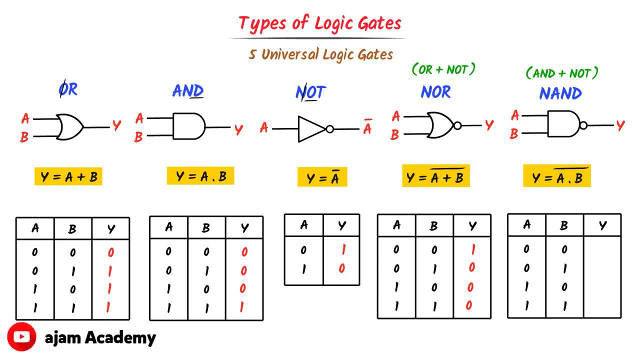 What about its truth table? Well, consider these possible values of a and b Now, AND gate will multiply them: 0 into 0 is equal to 0,. 0 into 1 is equal to 0,. 1 into 0 is equal to 0,. 1 into 1 is equal to 1.. While the NOT gate will inverse them. We know that. 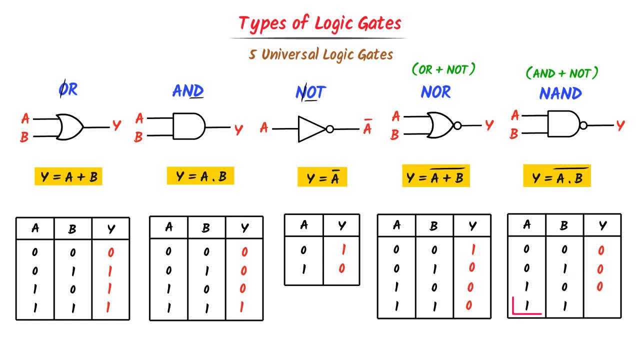 0 is equal to 0.. 1 into 1 is equal to 1.. While the NOT gate will inverse them, We know that inverse of 0 is 1 and vice versa. I write: 0 into 1 is equal to 0.. 1 into 1 is equal to. 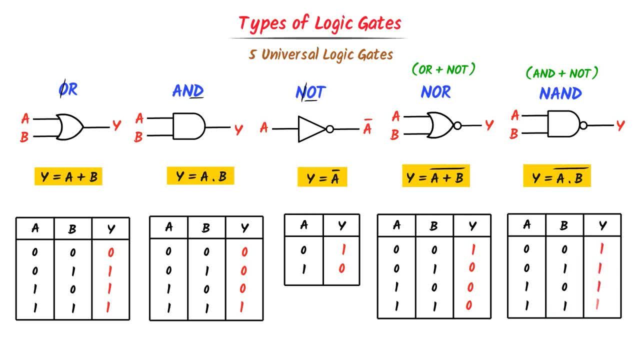 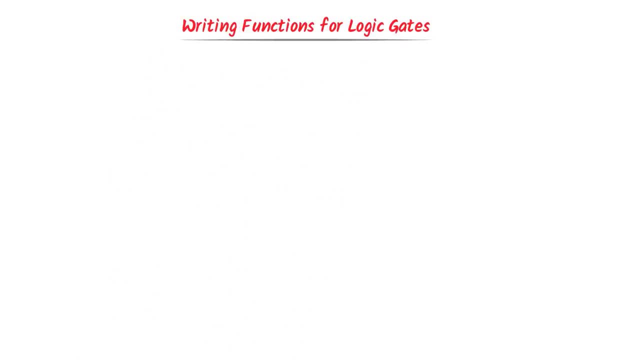 1. I write 1, 1, 1 and 0.. Hence, this is the truth table of NAND gate. Therefore, using this simple way, we can easily learn all logic gates. Now let me teach you that how to write function for any logic gate. Well, consider these two. 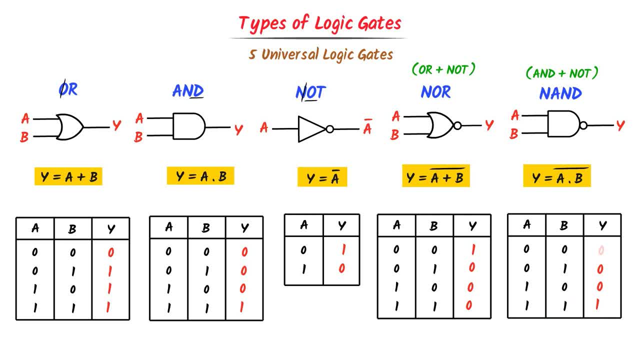 words of 0 is 1 and vice versa. I write 1, 1, 1 and 0. Hence, this is the truth table of NAND gate. Therefore, using this simple way, we can easily learn all logic gates. Now let me teach you that how to write function for any logic gate. 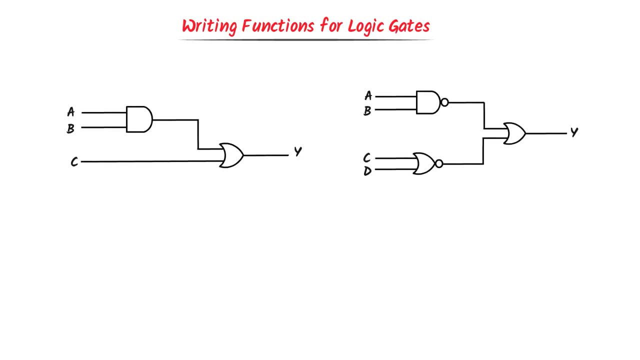 Well, consider these two systems. Firstly, I always spot the type of logic gate, For example, in the first system. this is AND gate, this is OR gate. Now two inputs, a, b, are given to AND gate. We know that AND gate will multiply the inputs, So we get a dot b as an output. Secondly, 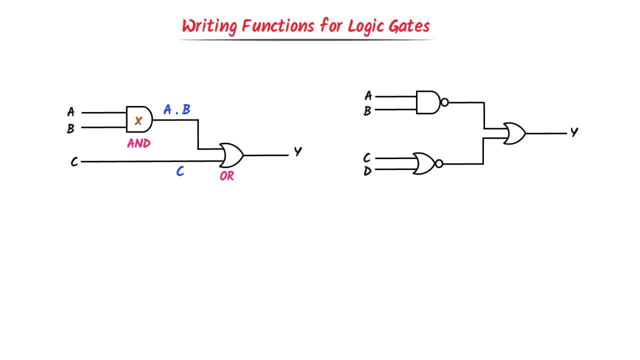 a dot b and this c is given as input to OR gate. We know that OR gate add the inputs, It adds a dot b plus c. Hence we get y equals a dot b plus c. On the other hand, this is NAND gate, this is NOR gate. 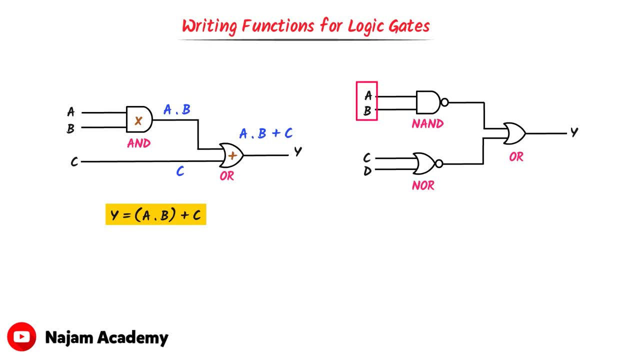 and this is OR gate. Now two inputs- a, b are given to NAND gate. The AND gate will multiply it- a dot b, While the NOT gate will inverse it. I put bar on a dot b. Secondly, two inputs- c, d- are given. 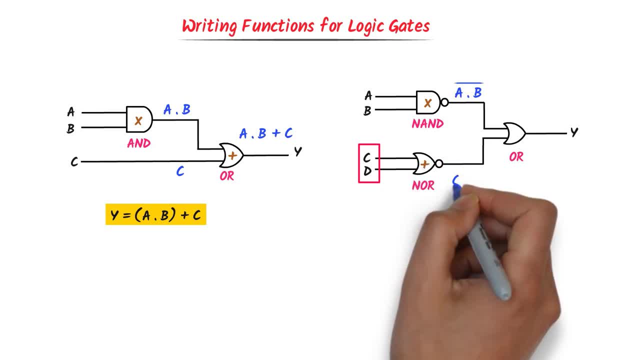 to NOR gate. We know that OR gate add the inputs. So we know that OR gate add the inputs. So we know that the OR gate will add it c plus d And the NOT gate will inverse it. I put bar on c plus d. 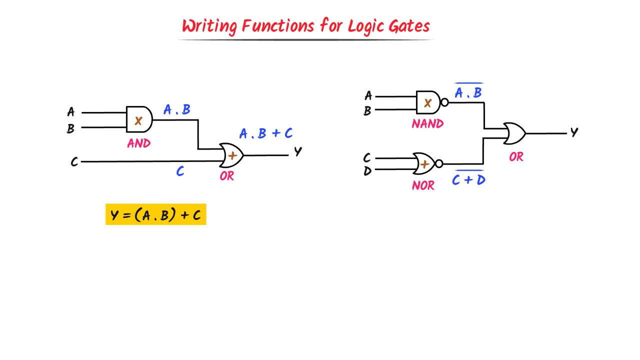 Thirdly, this OR gate receives two inputs: a dot b whole bar and c plus d whole bar. We know that OR gate will add the inputs. We get a dot b whole bar plus c plus d whole bar. Thus the function of this system is: y equals a dot b. 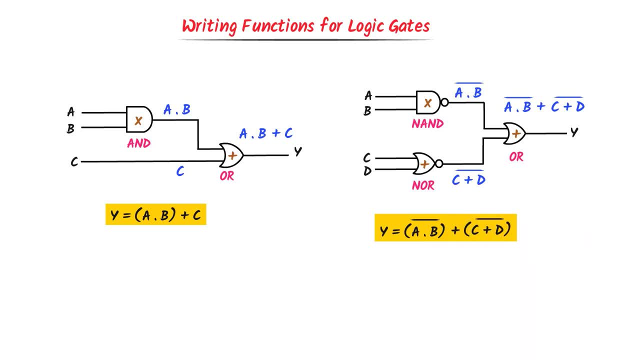 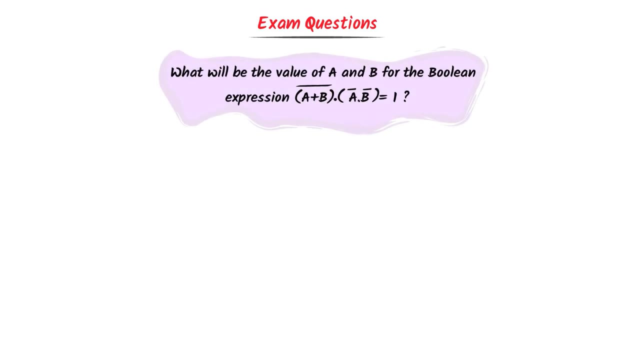 ab whole bar plus c plus d whole bar. Therefore, using this simple method, we can easily write function for any logic gate system. Finally, let me teach you some exam questions. What will be the value of a and b for the Boolean expression a plus b whole bar into a bar dot b? 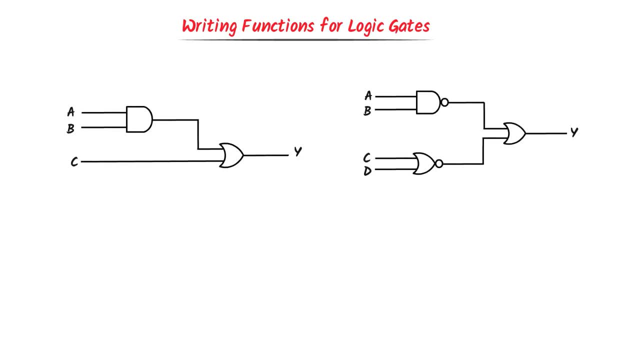 systems. Firstly, I always spot the type of logic gate. For example, in the first system. this is AND gate, This is OR gate. Now two AND ports a, b, are given to AND gate. We know that AND gate will. 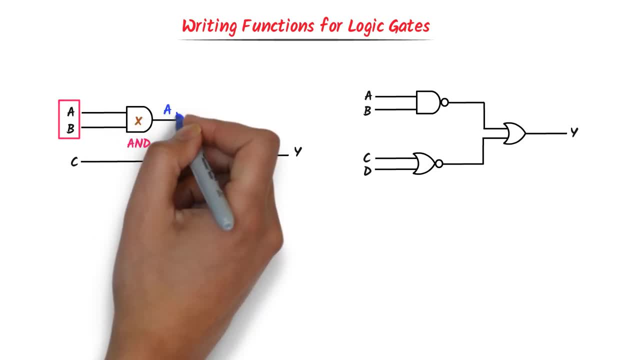 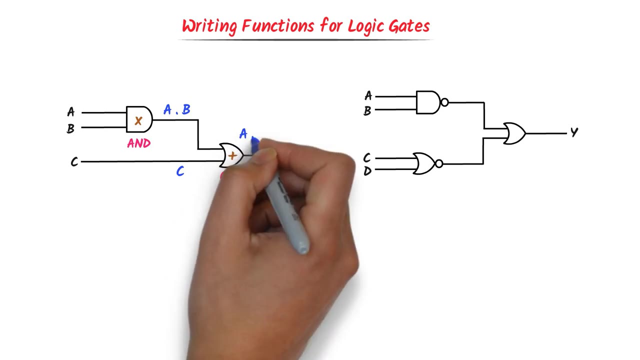 multiply the AND ports, So we get a dot b as an OUT port. Secondly, a dot b and this c is given as AND port to OR gate. We know that OR gate adds the AND ports. It adds a dot b plus c. Hence we get y equals a dot b plus c. 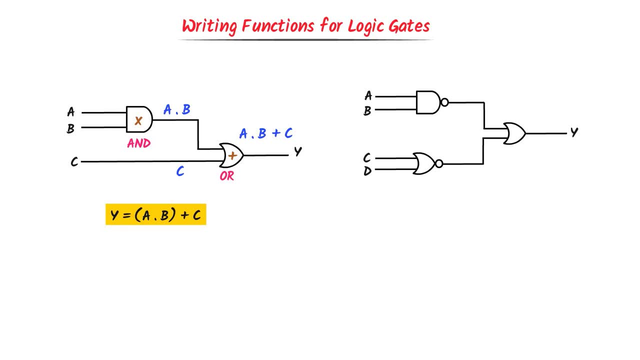 So we get a dot b plus c. Hence we get y equals a dot b plus c. Hence we get y equals a dot b plus c. On the other hand, this is NAND gate, this is NOR gate and this is OR. 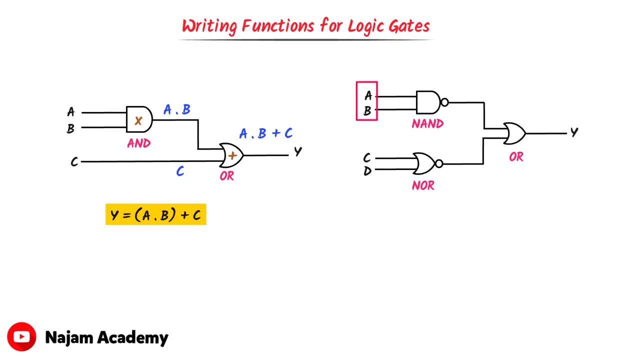 gate. Now two AND ports a, b are given to NAND gate. The AND gate will multiply it, a dot b, While the NOT gate will inverse it. I put bar on a dot b. Secondly, two AND ports c, d are given to NOR gate. The OR gate will add it c plus d And the NOT gate will add 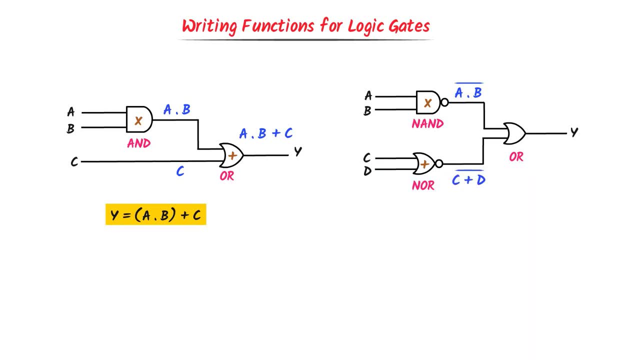 it c plus d. Here we have AND port, a dot b plus c plus d. Thus we get a dot b plus c plus d. Thirdly, this OR gate receives two AND ports: a dot b whole bar and c plus d whole bar. We know that OR gate will add the AND ports. We get a dot b whole bar plus c plus. 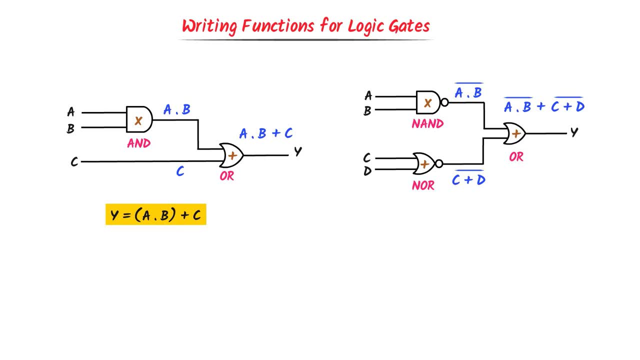 d whole bar. Thus the function of this system is: y equals a dot b whole bar plus c plus d whole bar. Therefore, using this simple method, we can easily write function for any logic gate system. Finally, let me teach you some exam questions. 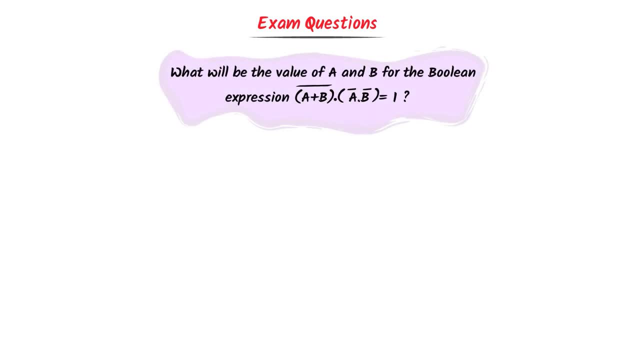 What will be the value of a and b for the Boolean expression a plus b whole bar into a bar dot b bar equals 1.. Well, the question is, what value of a and b should we take so that left hand side becomes equal to the right hand side? 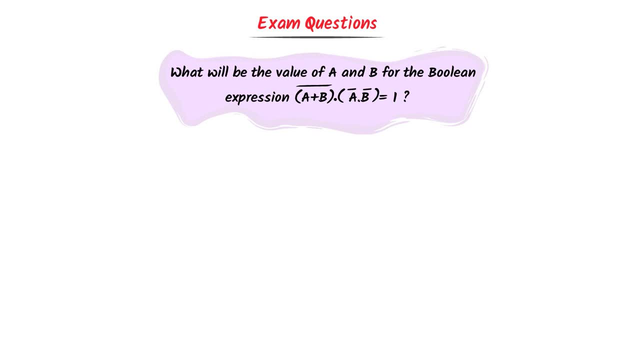 bar equals 1?. Well, the question is, what value of a and b should we take so that left hand side becomes equal to the right hand side? Let I take a equals 0 and b equals 0. Now consider left hand side, a plus b, whole bar into a bar. dot b bar. I put the values of a and b in it. I write 0 plus 0. 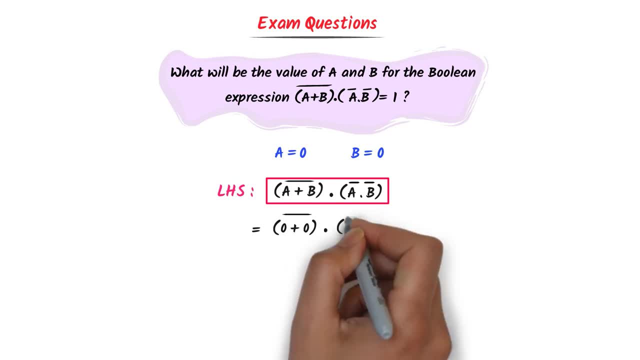 into whole bar: dot 0 bar, dot 0 bar. We know that 0 plus 0 is equal to 0. I write 0 bar and 2.. Also, we know that 0 bar, or inverse of 0, is 1.. I write 1 dot 1.. Now, this 0 bar means that inverse of 0, which is 1.. 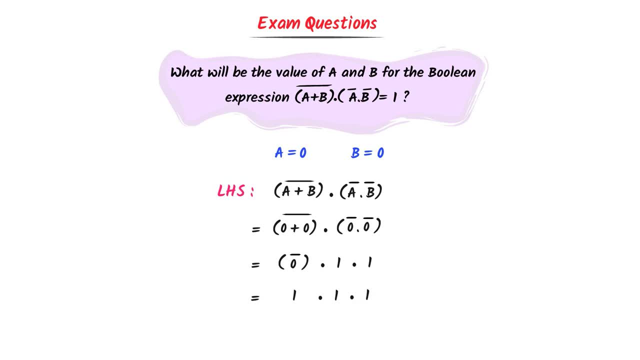 I write 1 dot 1 dot 1.. We know that 1 dot 1 dot 1 is equal to 1.. Therefore, if we take the values of a and b as 0, we get 1.. Hence, the value of a is 0 and the value of 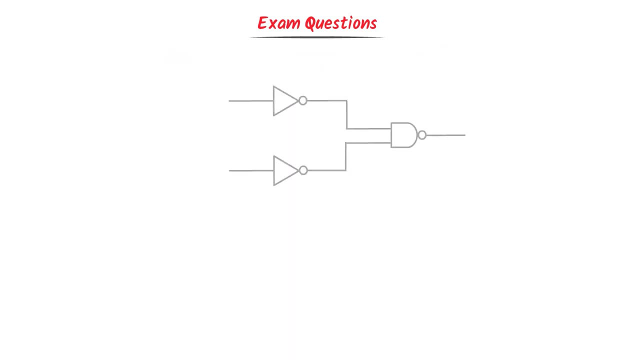 b is 0.. Secondly, consider this digital circuit. This logic gate is equivalent to dash. Well, firstly, I spot the logic gates. This is not gate, This is also not gate And this is nand gate. Now, this not gate will inverse the. 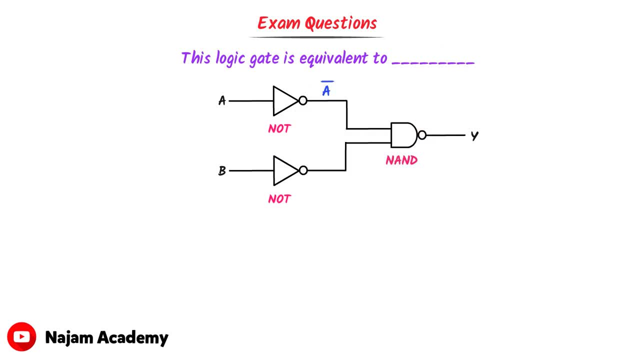 input A and we get A bar Here. we also get B bar. Secondly, this NAND gate receives two inputs: A bar and B bar. The AND gate will multiply it. We get A bar dot B bar, While the NOT gate will inverse it. We get A bar dot B bar into whole bar. Also, we know that. 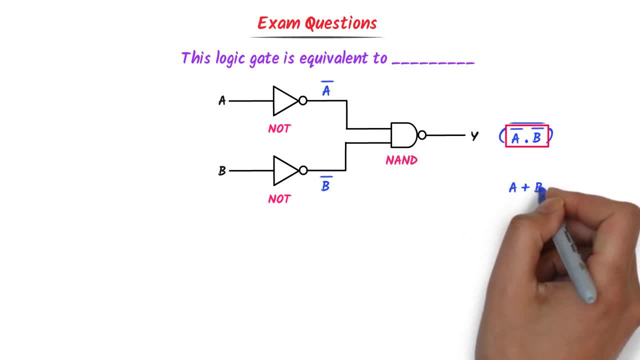 A bar dot B bar equals A plus B whole bar. So instead of this A bar dot B bar, I write A plus B whole bar. I get A plus B double bar. Also, we know that in case of double bars we cancel it. We get A plus B. We know that A plus B represents OR gate, Hence this digital. 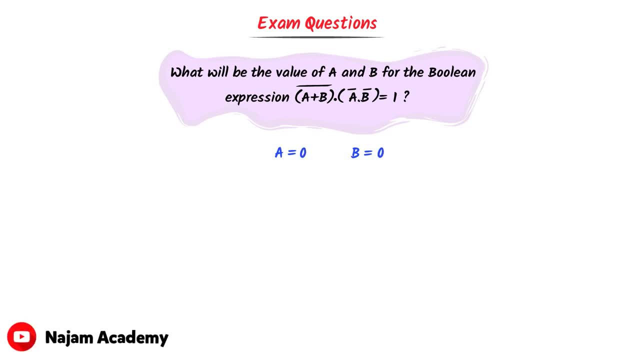 Let I take a equals 0 and b equals 0.. Now consider left hand side: a plus b, whole bar into a bar, dot b bar. I put the values a and b in it. I write 0 plus 0 into whole bar, dot 0 bar. dot 0 bar. 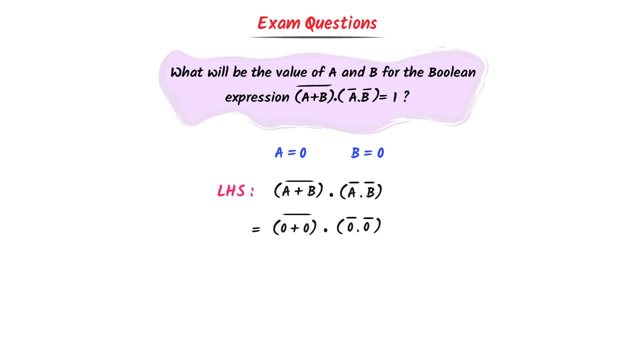 We know that 0 plus 0 is equal to 0.. I write: 0 plus 0 equal to 0.. Well then, let's Calculate the problem: 0 bar and 2.. Also, we know that 0 bar, or inverse of 0, is 1.. 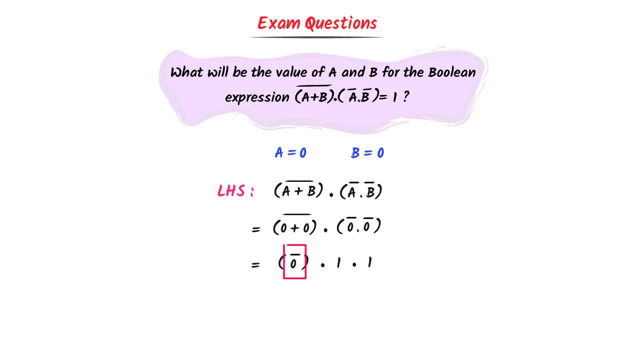 I write 1.1.. Now this 0 bar means that inverse of 0, which is 1.. I write 1.1.1.. We know that 1.1.1 is equal to 1.. Therefore, if we take the values of a and b as 0, we get 1.. 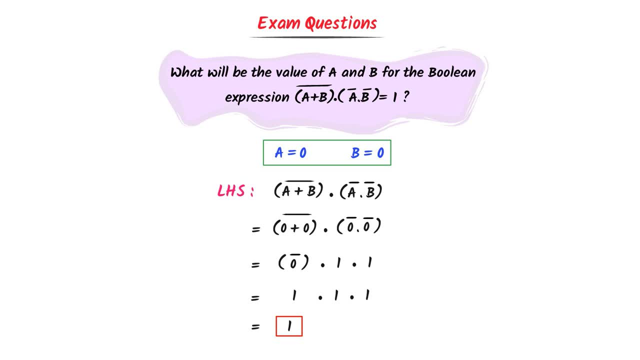 Hence, the value of a is 0 and the value of b is 0.. Secondly, consider this digital circuit. This logic gate is equivalent to dash. Well, firstly, I spot the logic gates. This is NOT gate, this is ALSO NOT gate and this is NAND gate. 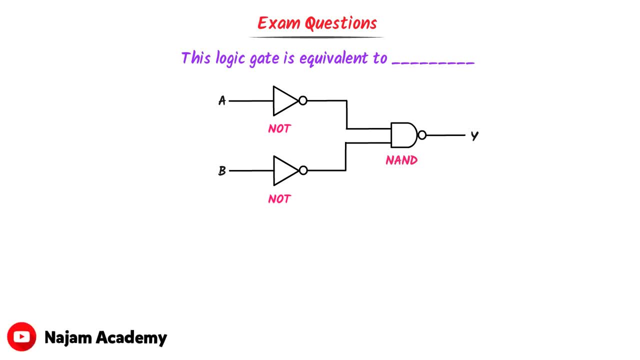 Now this NOT gate will inverse the input a and we get a bar Here we also get b bar. Secondly, this NAND gate receives two inputs: a bar and b bar. The AND gate will multiply it. We get a bar dot b bar. 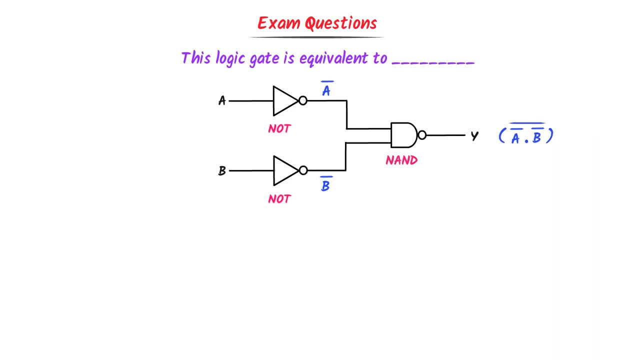 While the NOT gate will inverse it. We get a bar dot b bar into whole bar. Also, we know that a bar dot b bar equals a plus b whole bar. So instead of this, a bar dot b bar, I write a bar dot b bar. 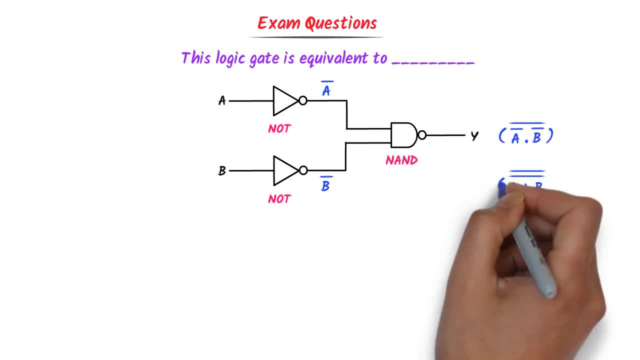 I get a plus b double bar. Also, we know that in case of double bars we cancel it. We get a plus b. We know that a plus b represents OR gate. Hence this digital circuit is equivalent to OR gate. Thus, using this simple method, we can solve logic gate problems easily. 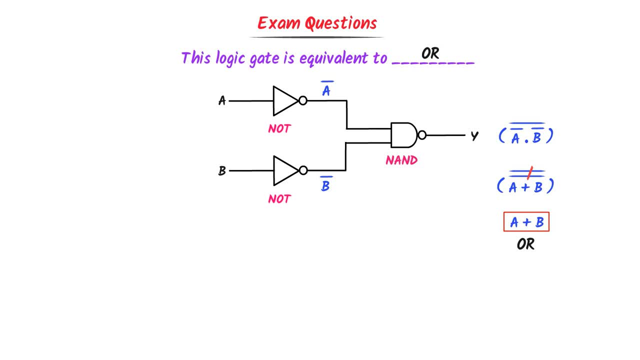 I hope that you have learned all about logic gates.